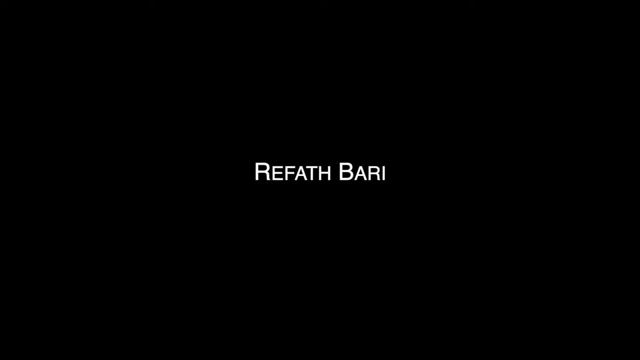 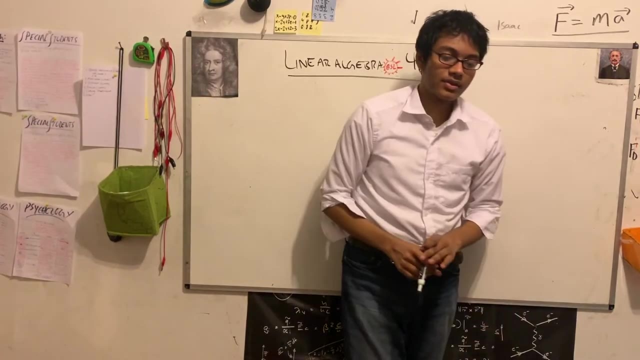 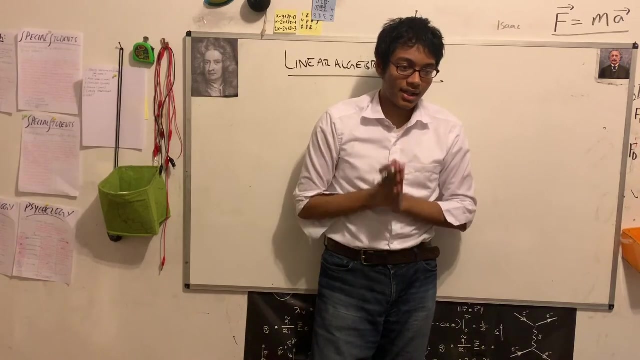 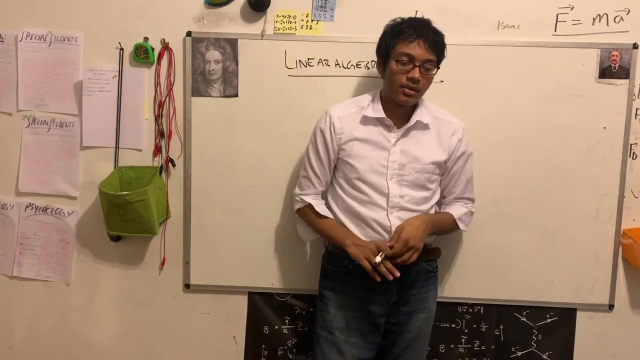 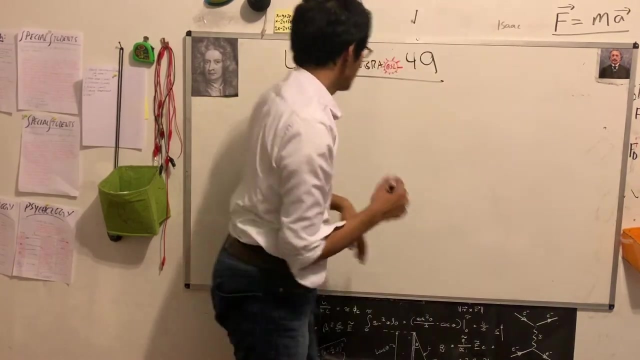 Dream to become the next Sir Isaac Newton or Albert Einstein. Learn from the master Raphat Bari. Watch his videos to achieve your dream. So, uh, let's get started with the do now. okay, So we celebrate because we're at half a hundred. 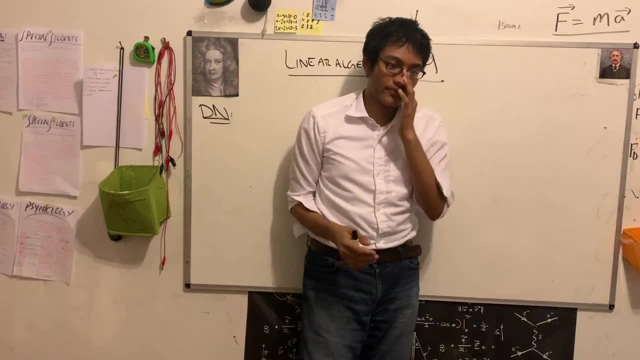 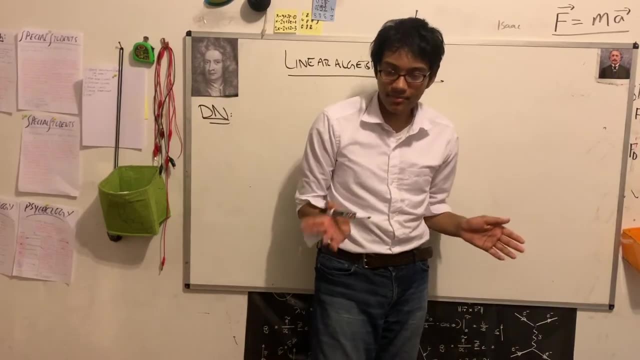 Here. So today's idea is gonna kind of treat matrices just like numbers. So just like you can add numbers, you can add matrices. Just like you can multiply numbers, you can multiply matrices. So today we're gonna take the concept of multiplication further. 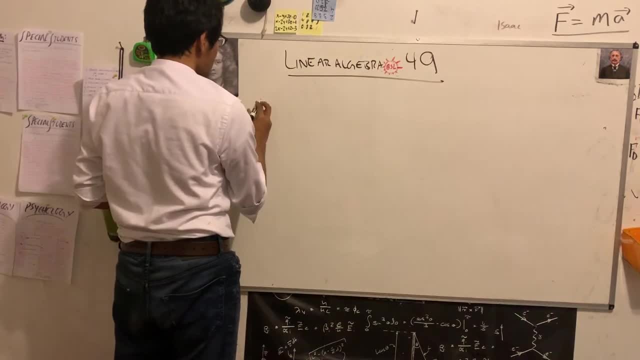 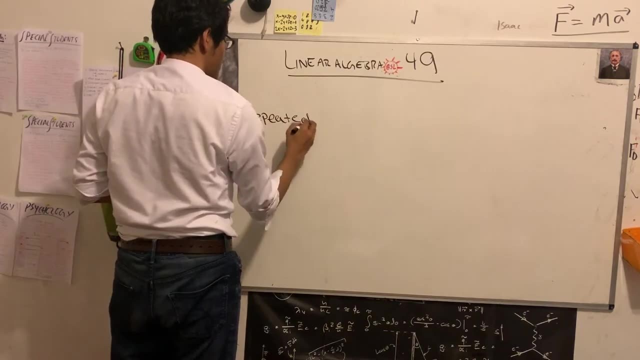 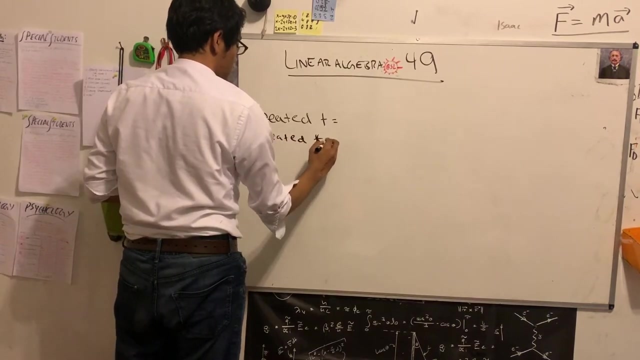 Okay, So let's see. Um, let me. And why don't matrix exponents exist? Uh, okay, Well, hopefully this will serve you. Oh, Okay, so I put the word right out of my mouth. I talk with this about. I talk about this with a friend. 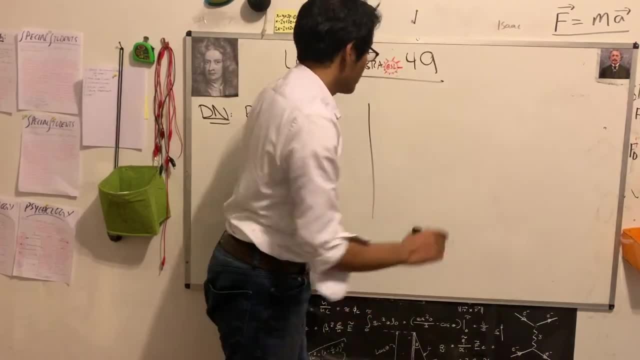 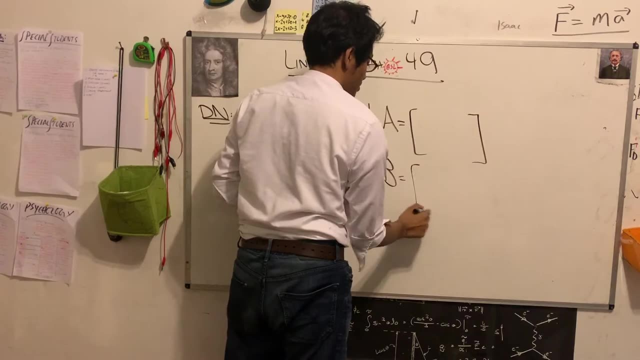 Right, Yeah, Okay, good, good, good, Okay. so I'm gonna give you two matrices. I'll call them A and I'll call them B, okay, So, okay, these are extremely random matrices and I want you, I want you to do what. 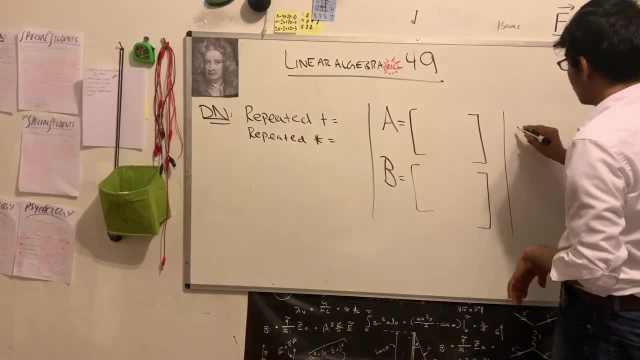 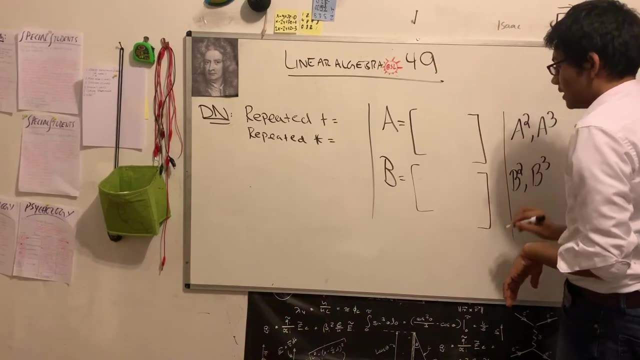 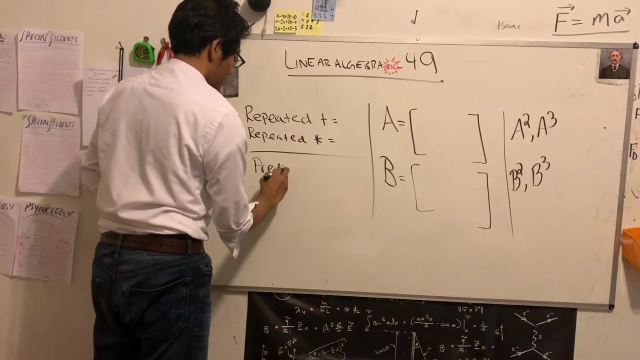 I'll tell you what. Um, I guess, I'll ask you to find a squared and a cubed, and find b squared and b cubed, and then I'll ask you to do one final thing, and that is this: predict, predict, predict. 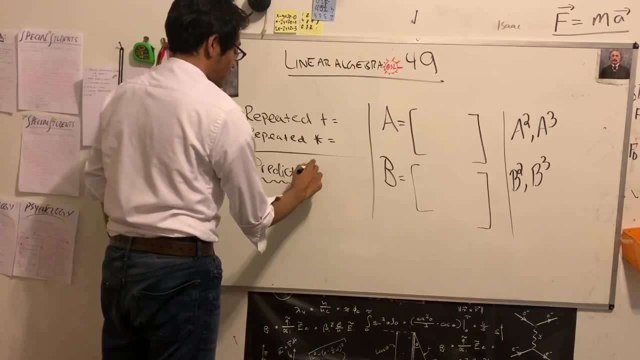 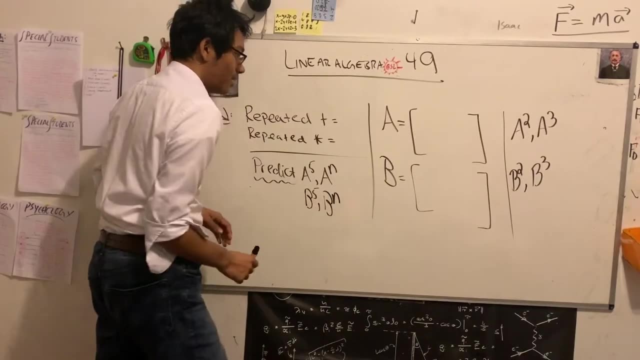 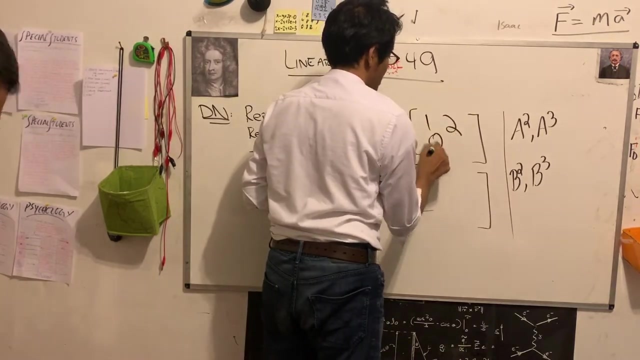 LS3, You don't have to say: predict so many times a to the 5,, a to the n, Yeah, And b to the 5, and b to the n, okay. So there you go, go ahead. but you can't do anything because there's no numbers here. so let me put in the numbers. 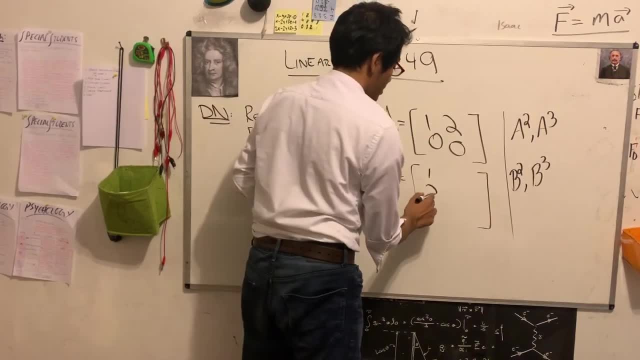 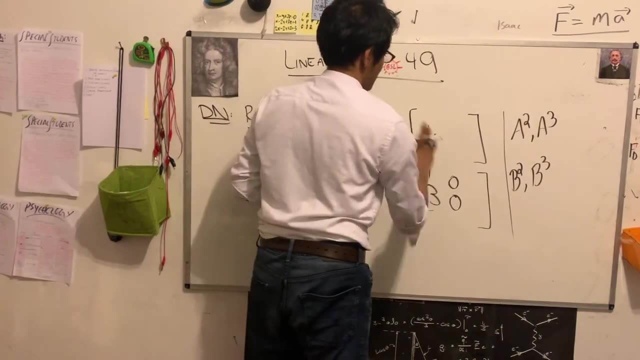 Those are definitely random. Yeah, they're very random, Super random. Okay, so why don't you guys? okay, whoa, whoa, whoa, whoa, whoa whoa. Let's not try to sabotage my lesson here, okay. 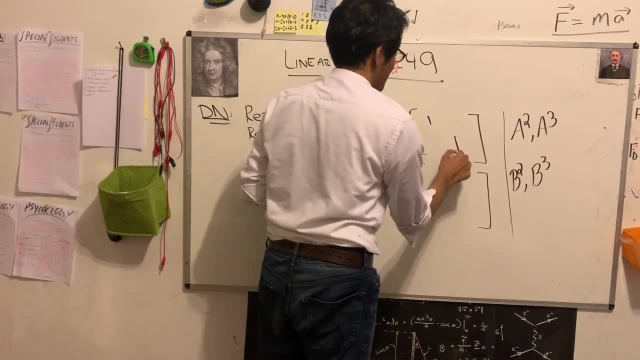 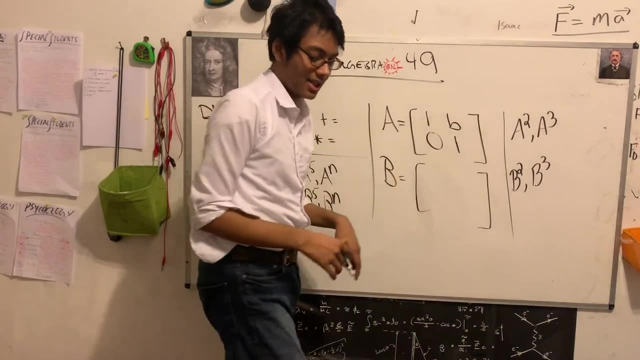 Before I get started, I want you to look for any patterns in the matrices I'm going to give you. okay, Wait, what if it's number b? This b can be any constant. okay, Any constant at all. That's the do now. 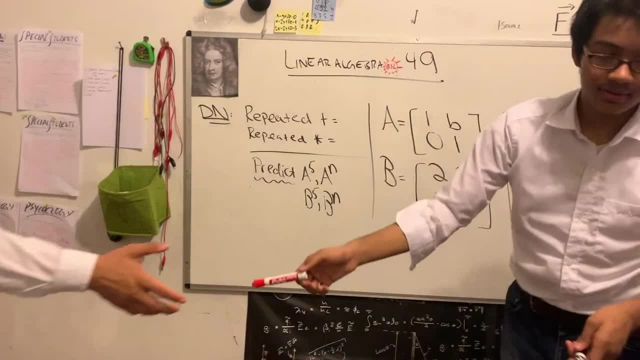 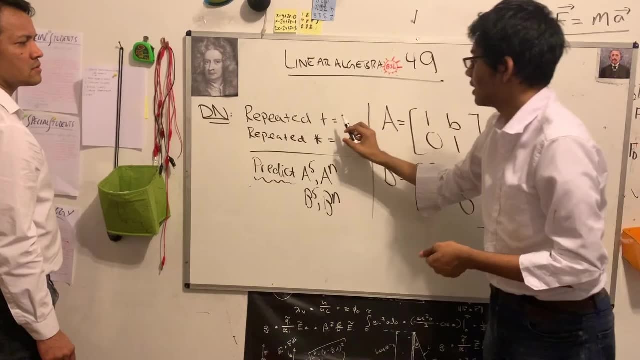 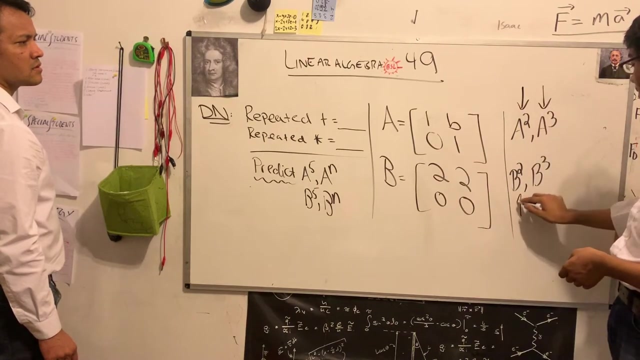 Yeah, this is the do. Okay, Go ahead and try your best. So all we need to do is create b. No, what is repeated multiplication equal to, Repeated multiplication equal to? And you can do the first- a squared and a cubed- and, as I said, we'll do b squared and b cubed. 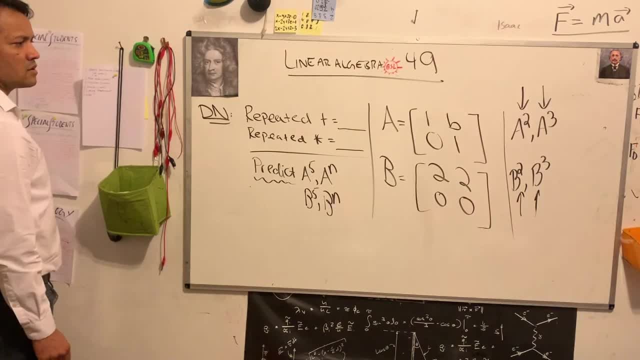 But b is not there. how can you do that? Oh, here it is. No, I mean this one. Huh, The b is unknown. Yeah, it's general. So what is it? 1 or 0?? 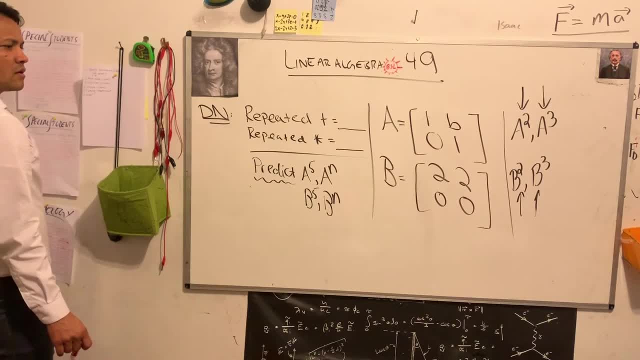 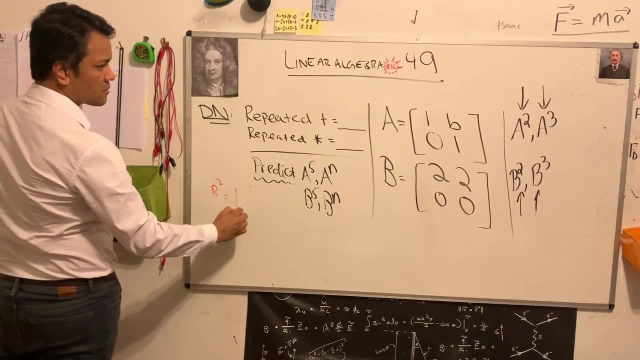 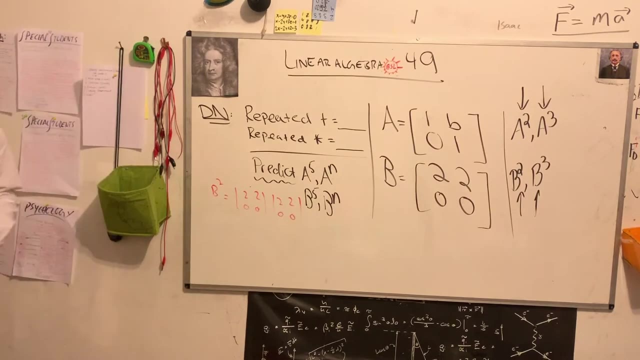 It's any number, Any number, So I'm going to do this one. Okay, b squared is equal to 2, 2, 0, 0, 2, 2, 0, 0.. Oh, so no answer. 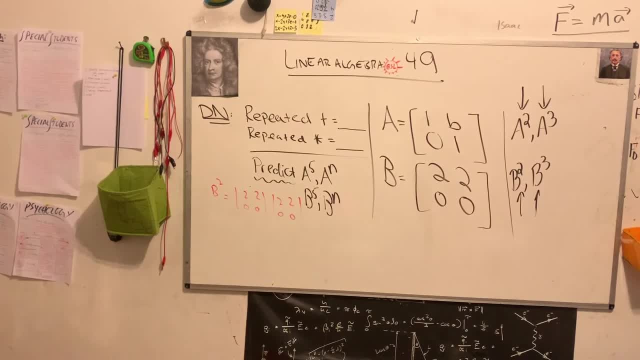 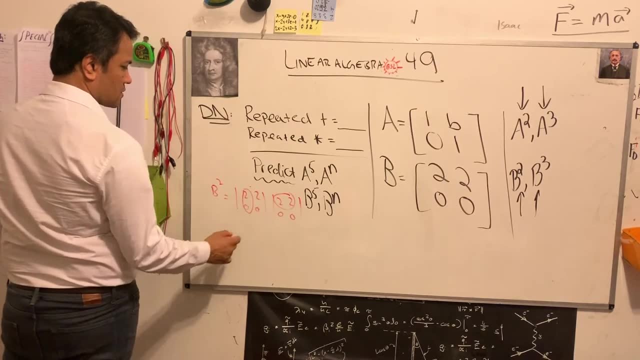 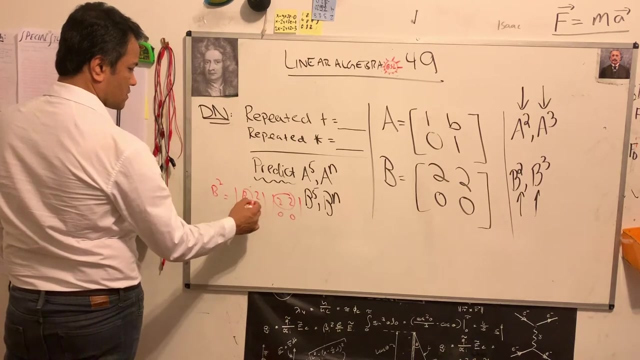 No, you have to multiply it. So you have to multiply it. okay, sure, I'll do that. This is a mix of the two methods, right? No, this isn't. So can you give me the number of the first and the number of the second? 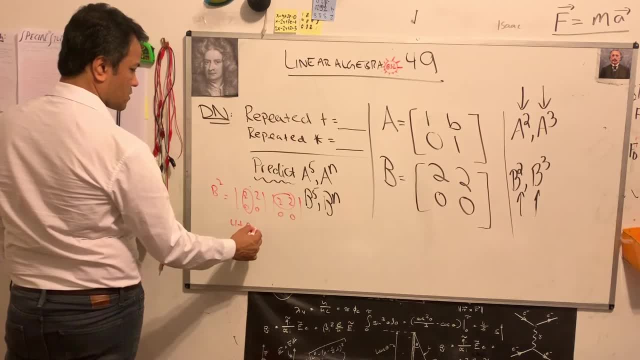 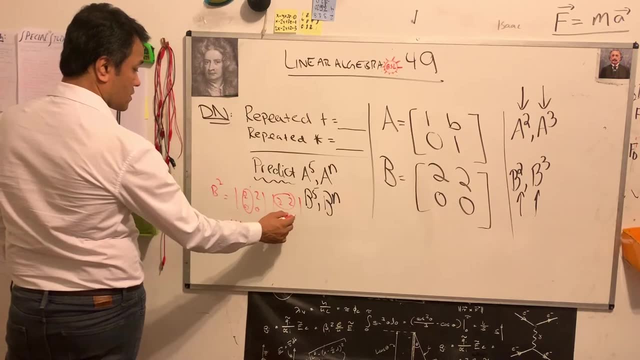 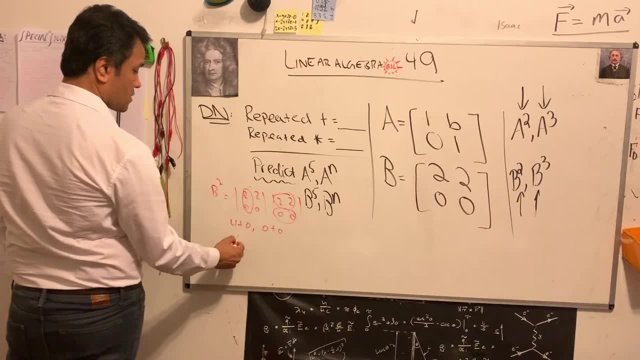 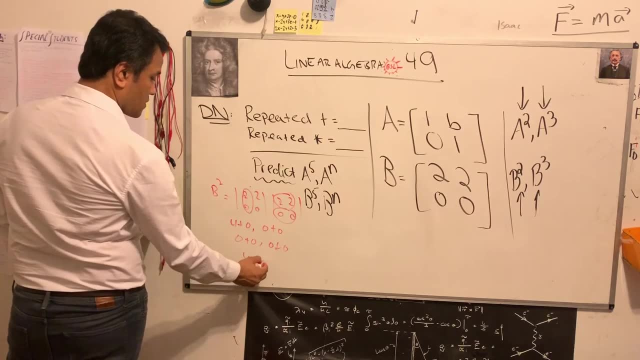 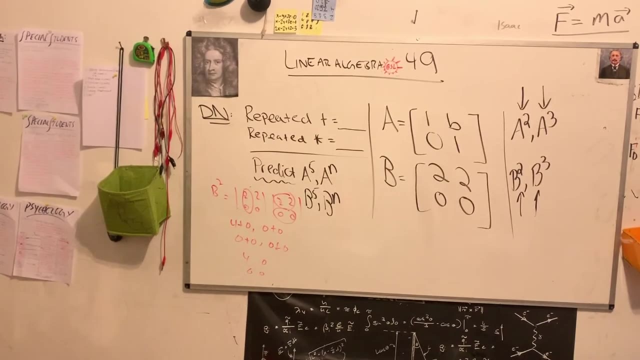 Is that correct? Is that correct? Ok, What's your answer? b b. No, this isn't b squared: 0. 0. 0.. to a square. so this is kind of hard because we have some general constants here, but that's. 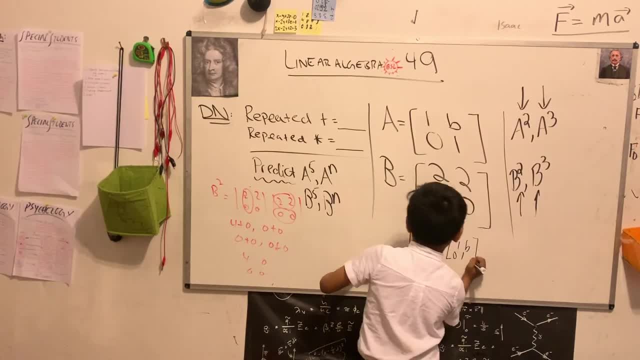 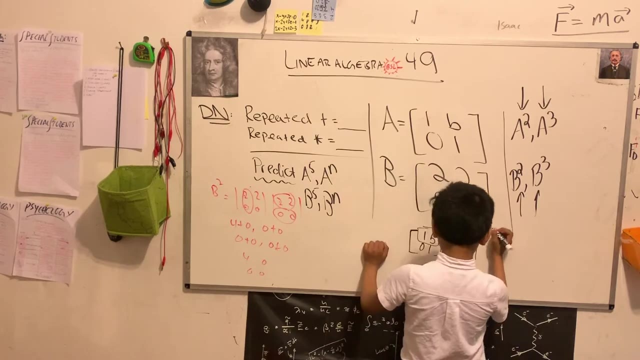 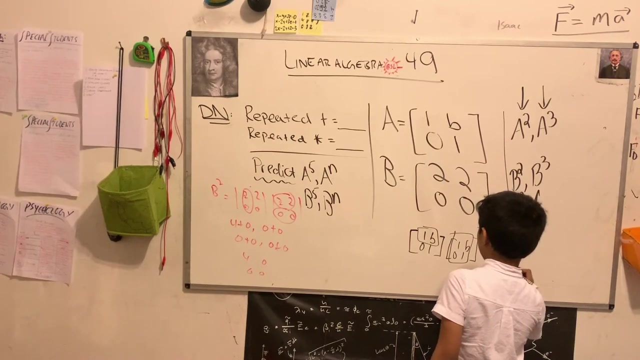 going to be O1.. So we can read right to left, and I'm choosing the broken way, So I take this and multiply it by this. So we want 1 of the first row and B of the second row. 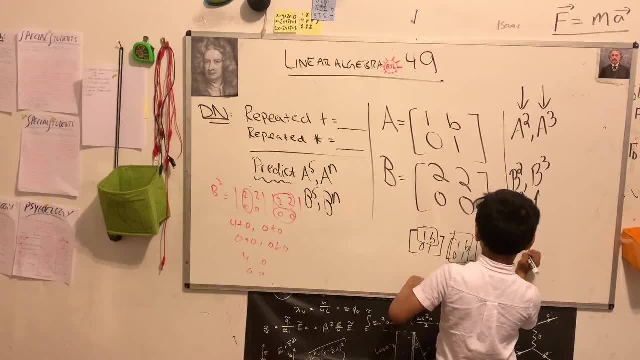 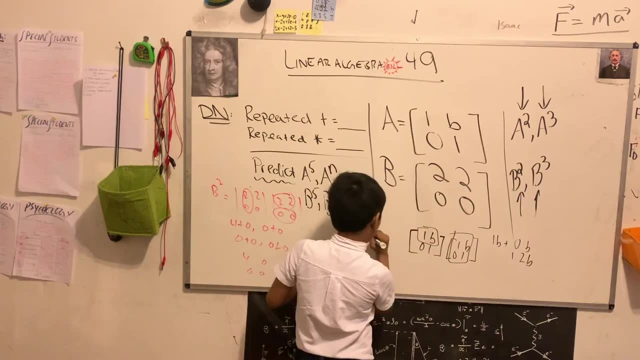 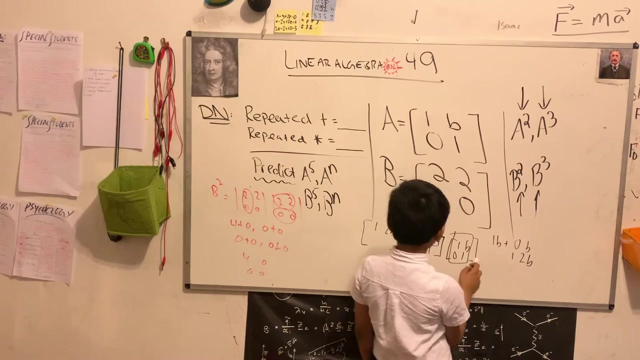 So 1B plus 0B, so that would give us 1 and 2B. So that would give us 1 and 2B. So that would give us 1 and 2B, Then 0, 1, so we want 0 of the second row plus 1 of the second row, so that would be. 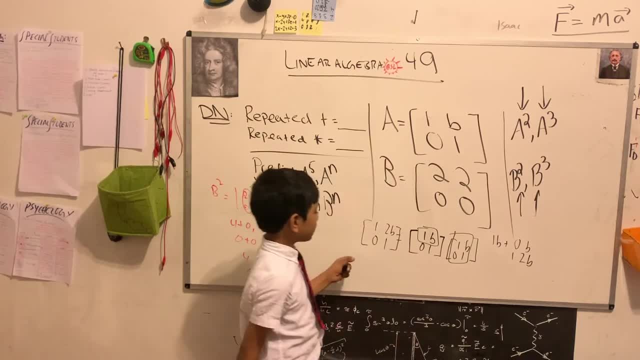 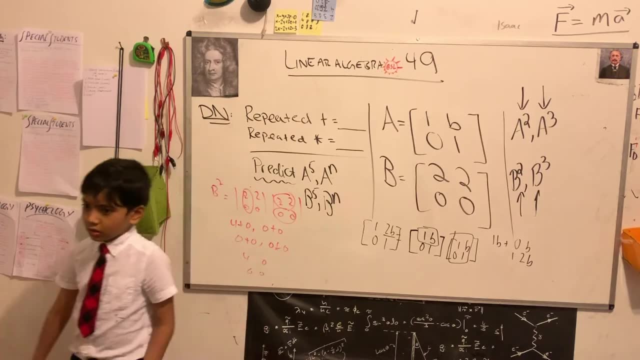 0, 1.. 1, 2, B: 0, 1.. So I notice that the number, all the numbers, this number doubles. Okay, okay, Strange, weird, complex. You want to predict what A to the 5 is. 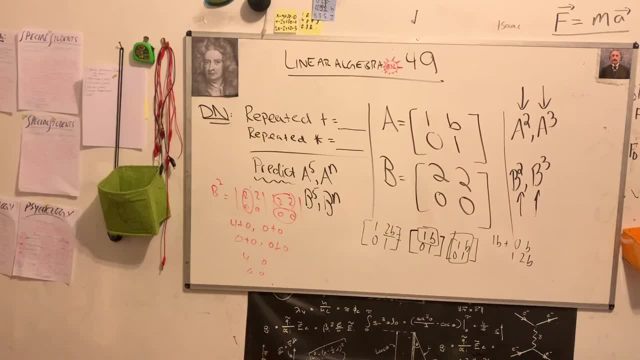 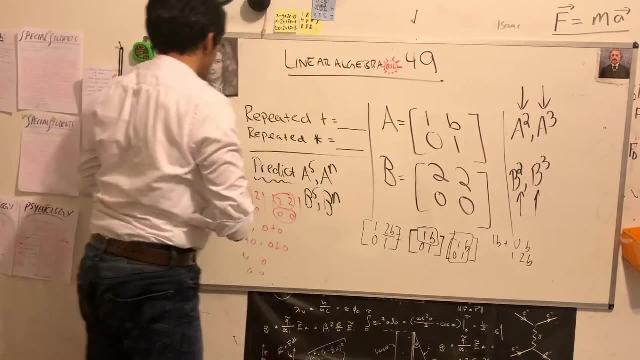 Hmm, Hmm, Hmm, Would that be 1, 5, B, 0, 1? Okay, so, adios, No, Give me your marks, Give me your marks. So, as part of our lesson, we are going to try to verify our students' answers, okay. 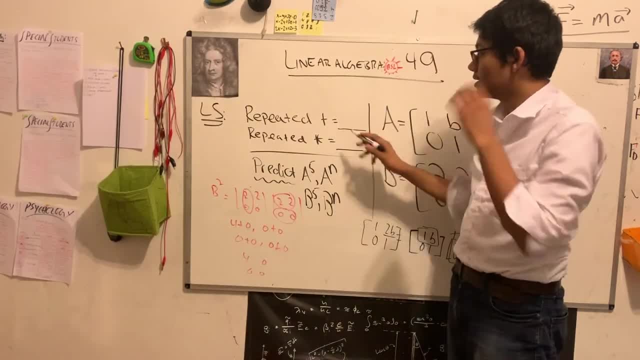 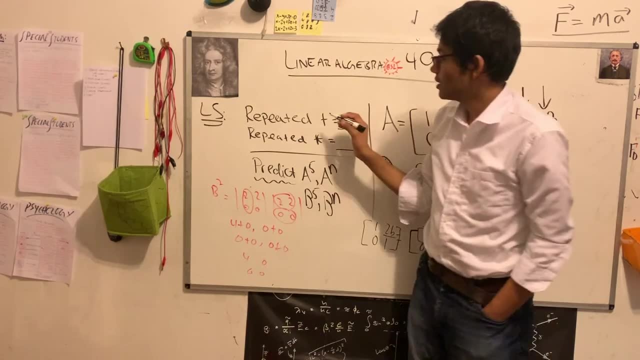 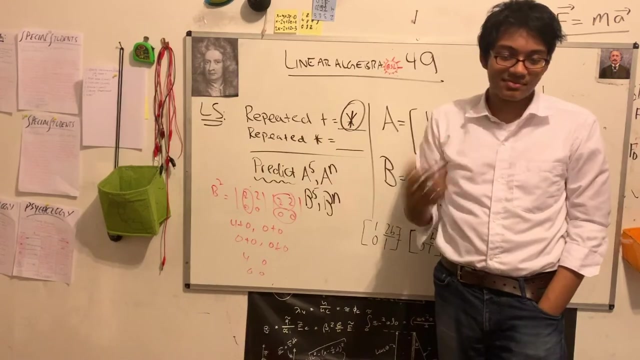 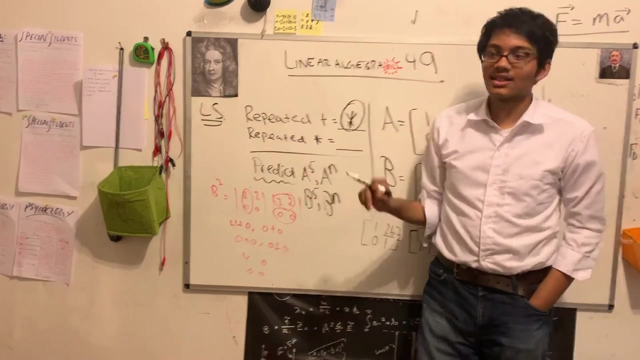 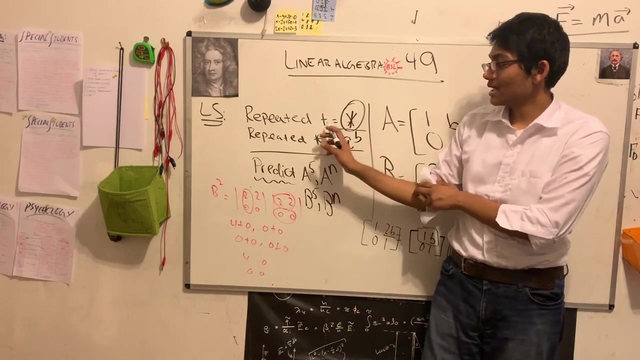 But before we verify anything, I want to start with this. When I add the same number to itself multiple times, what does it become? Multiplication, right? So repeated addition is multiplication. So repeated multiplication is Exponent, Exponent, Exponent. And it turns out we can. can we multiply matrices? can we add matrices? 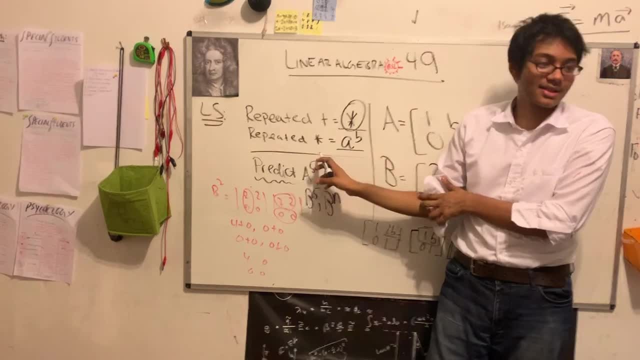 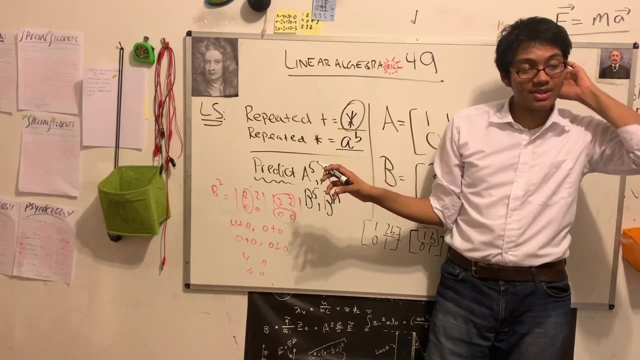 Yeah, Yeah, That means we can multiply matrices. We've been multiplying them for the last. Oh, that means we can do the exponential. We can do exponents with matrices, right, So that's pretty good. We've been multiplying them more like a multiplicator. 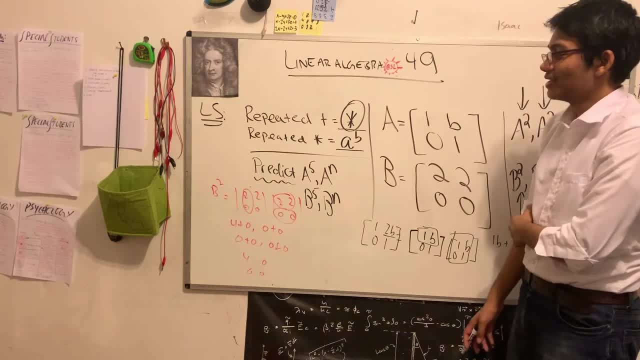 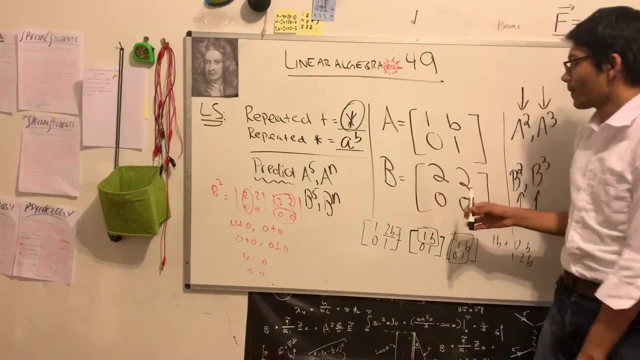 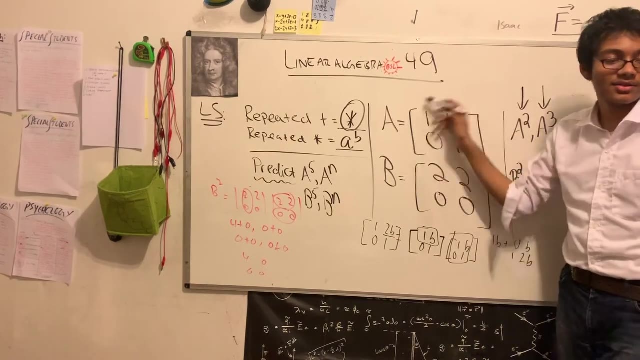 find them for like the last 20, last 20, like that. so now we're gonna try to find the exponents, the powers of matrices. okay, so, okay. so, let's see, uh, we're gonna begin with a matrix. a what kind of matrix does this look like to you? okay, uh, once we look at the wall, he's fairly confused. but what? 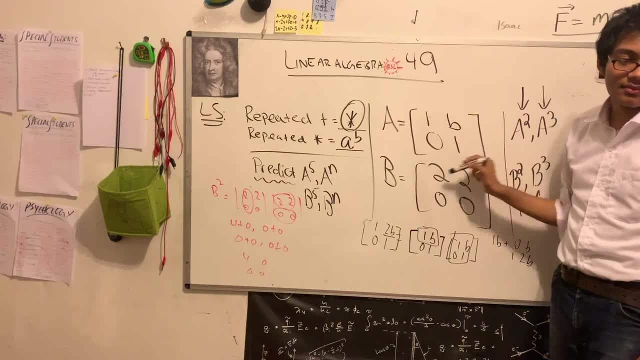 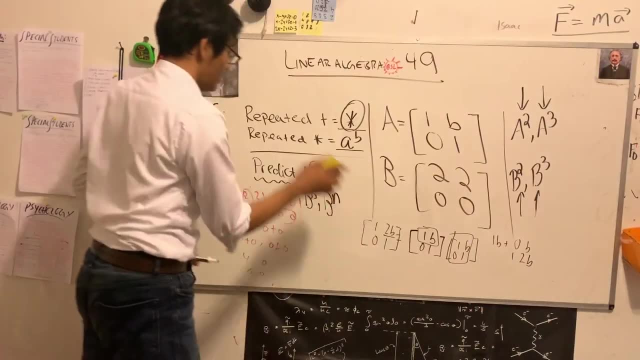 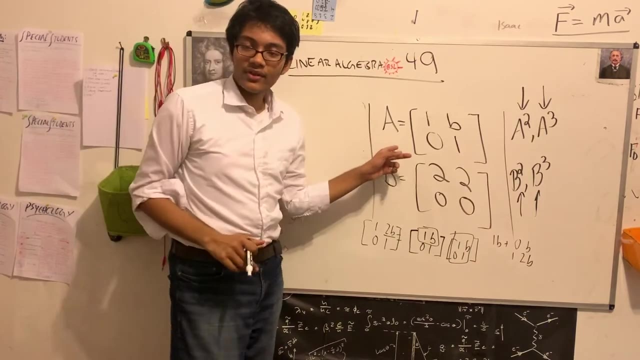 does panda matrix? does this look like to you? uh, this looks like an identity, except one of the zeros is replaced with a constant. well, everything is the same, except the constant is doubled, right? so if i uh create this part, then let's see. our student found out that if i multiply this matrix, 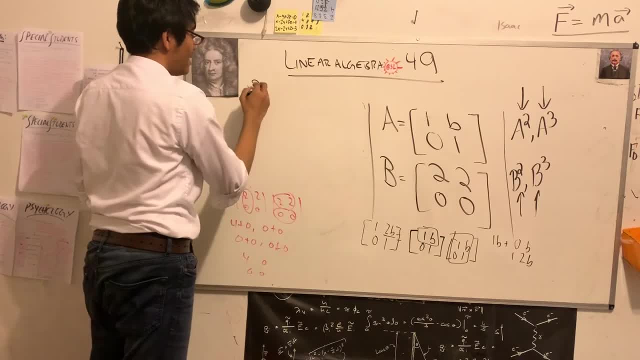 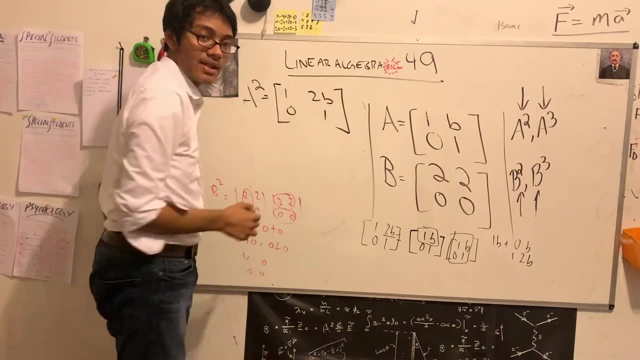 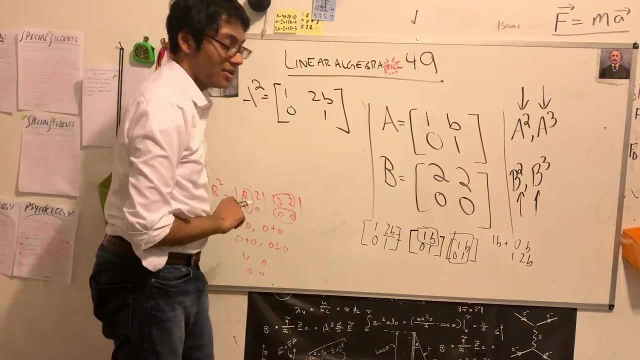 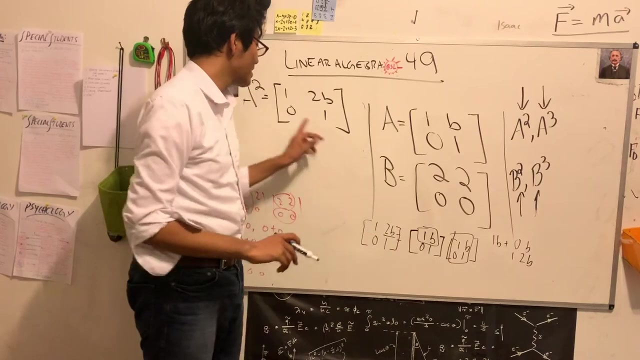 by itself. in other words, if i have this identity matrix and i square it, i'm gonna get one to be zero, one, right. everything doesn't change except, yeah, that's double. that's very weird, do you know why? because when we do the dot product weight, these zeros have a way of canceling out any extra time. okay, so yeah, because you want zero with the. 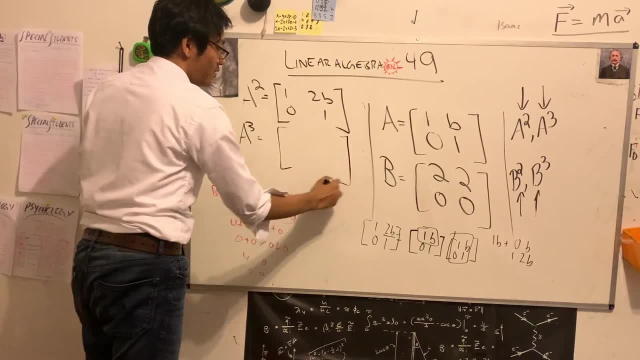 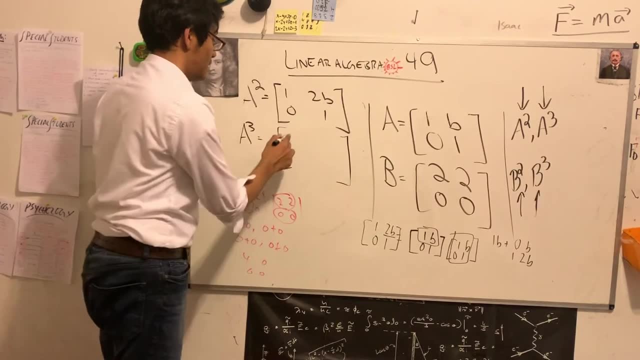 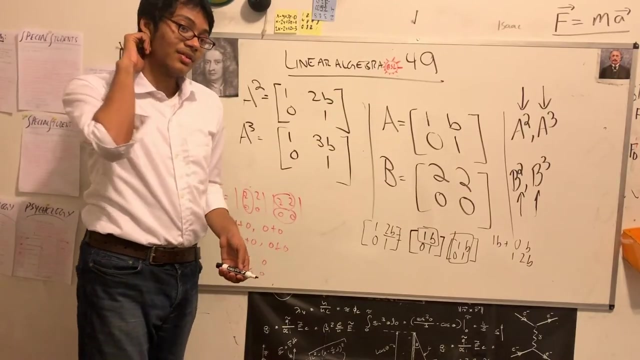 first one, yeah, yeah. so what do you think a cubed will look like? so a two would look like one. three b, zero, one, right, yeah. so now it's kind of an obvious pattern. it's because- oh no, i wasn't watching. oh, wait it- because if you kill, if you put one or zero to any 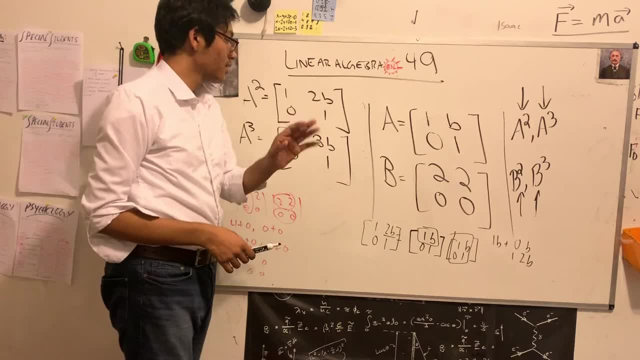 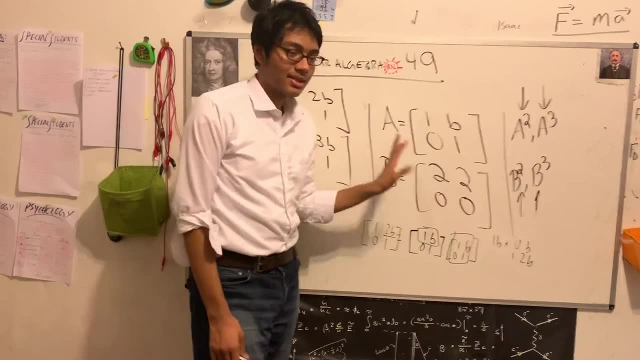 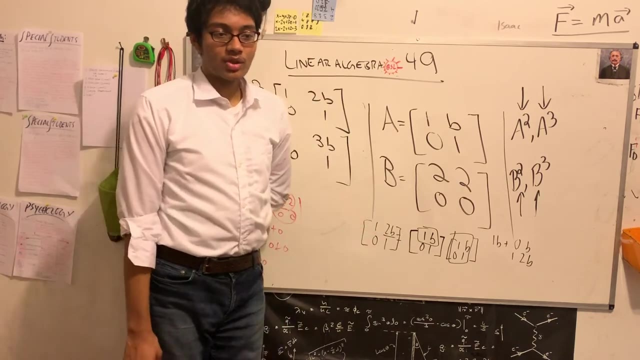 x point, it'll become itself. but okay, okay, any certain number. good, so it doubles and triples. can you explain it again? yeah, so let's, let's see what we just did. we told ourselves that we can multiply matrices. right, so if we can multiply matrices, we should be able to find their powers. 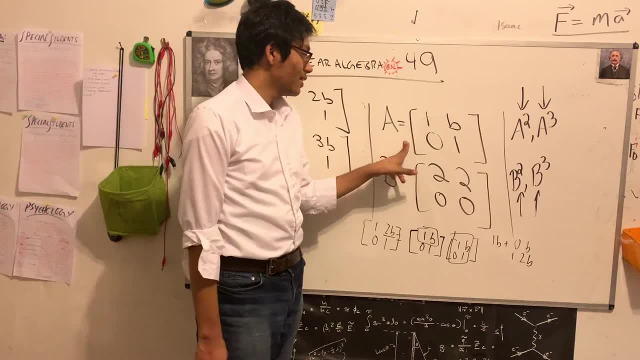 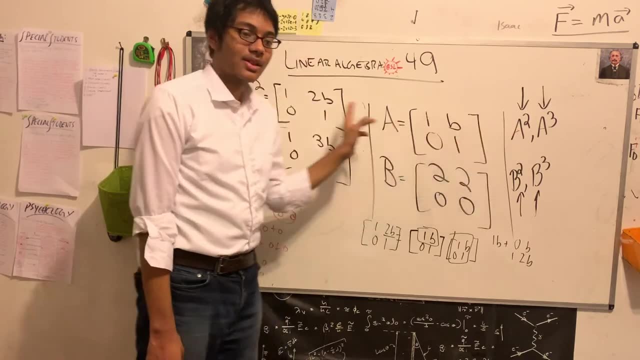 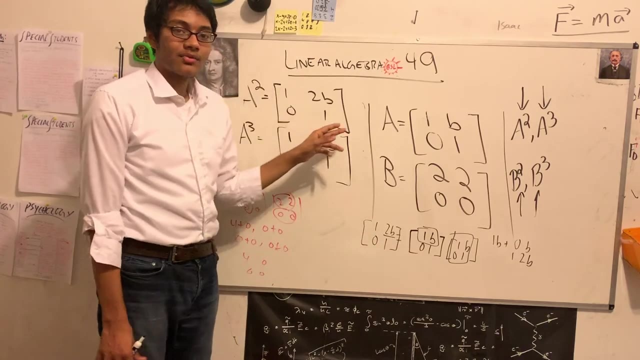 so if i have a, if i have a, if i have a identity matrix- one b, zero, one right- and i want to find the square of this matrix, all i have to do is multiply the matrix by itself. that's what our student read here and he found that there is a pattern when you multiply this. 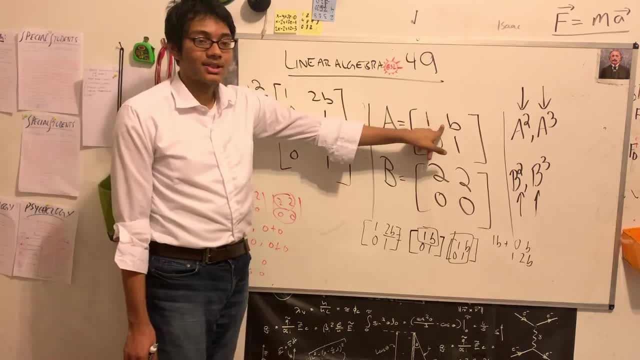 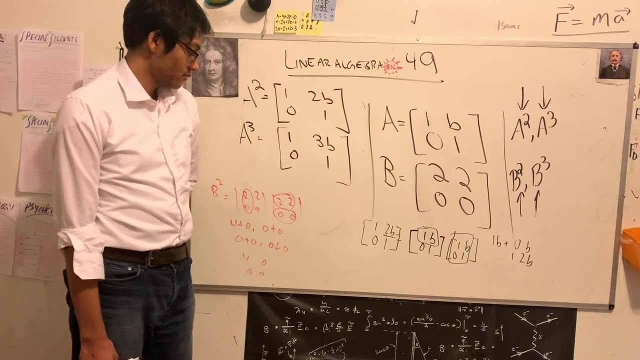 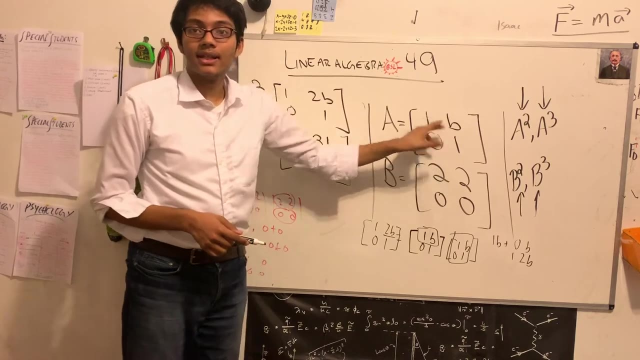 identity matrix by itself constant changes. so why you don't write? well, if you multiply b times b, you get uh b squared, so why don't you? why did you write two b? no, this is the result. uh, this is for uh a. this is for a. this is for matrix a. this b is completely different from this b. 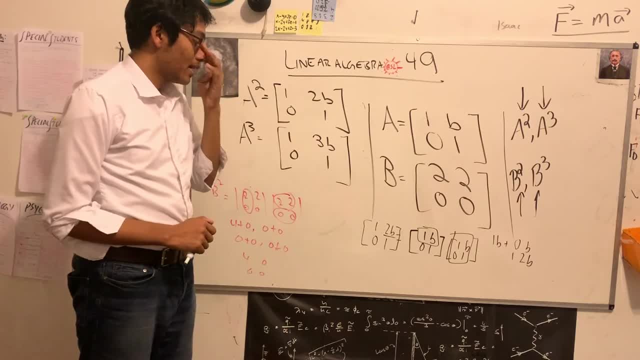 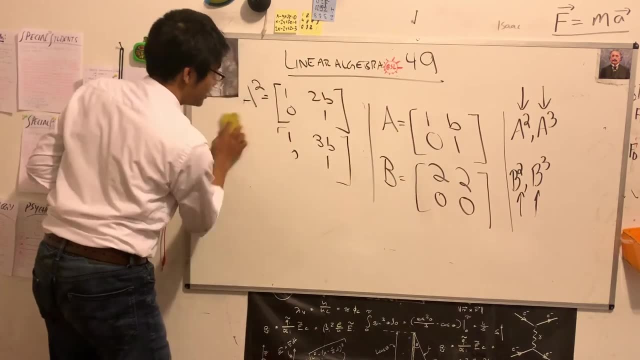 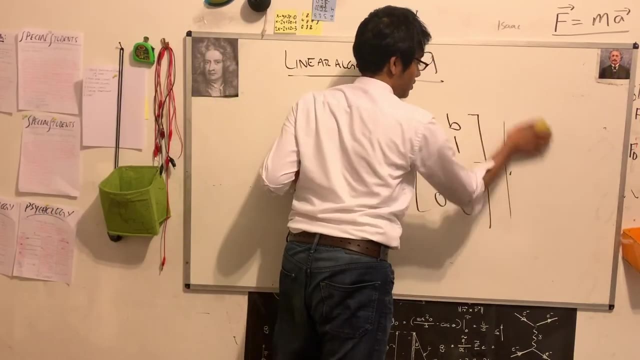 no, oh that you said you have to multiply by, yeah, so okay, yeah, let me show all the steps. okay, really, i'll show all the steps. it's gonna become very clear and very nice, really, yeah, okay, oh yeah, i'm just gonna sleep doing this portion. you're gonna help us if we get it started. so i have this matrix right, yeah, i have a matrix. 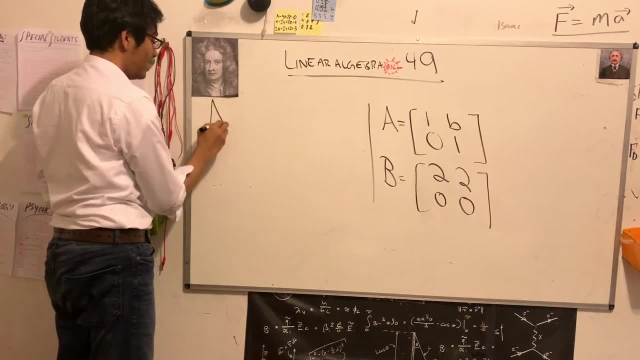 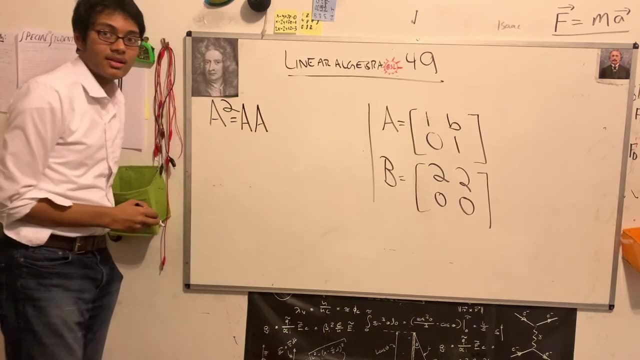 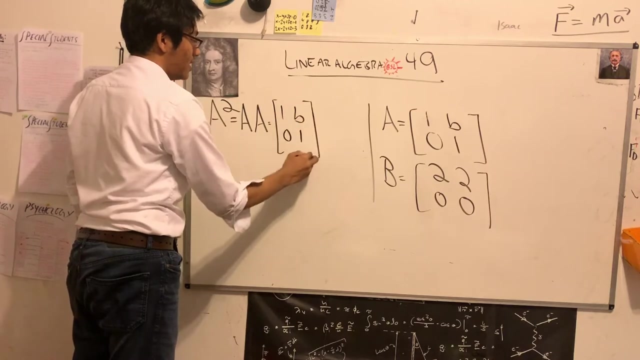 let's call our matrix a. my goal is to find a squared, so a squared is the same thing as you're trying to say. of course, a is just one b zero one, and a is once again just one b zero one, right, yeah? so now what i'm going? toets you. 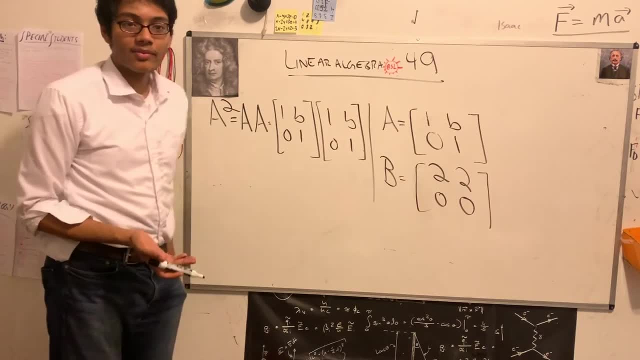 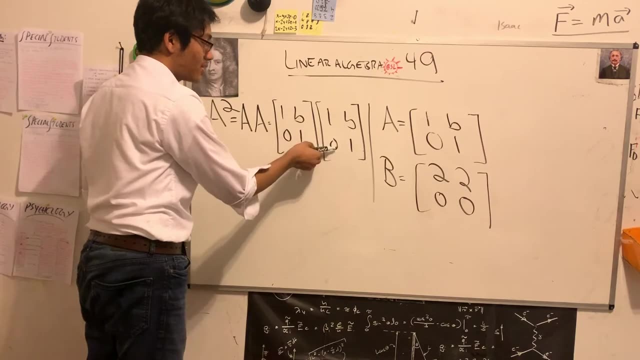 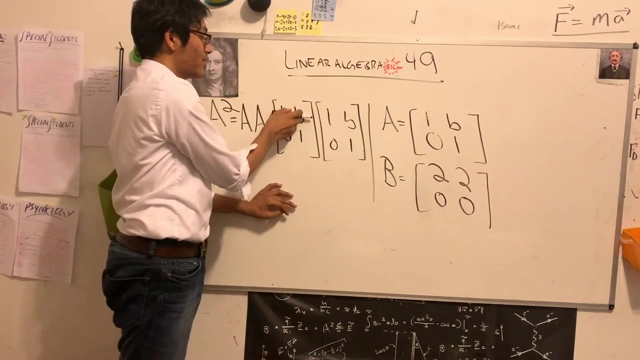 so now what i'm going toets you to do is i have three different options for multiplying, because i've shown you all the different options over the last 20 lectures. i can do row times column. uh, during the do now you did column times row, but that's illegal. we, when we do the dog product way, we always have. 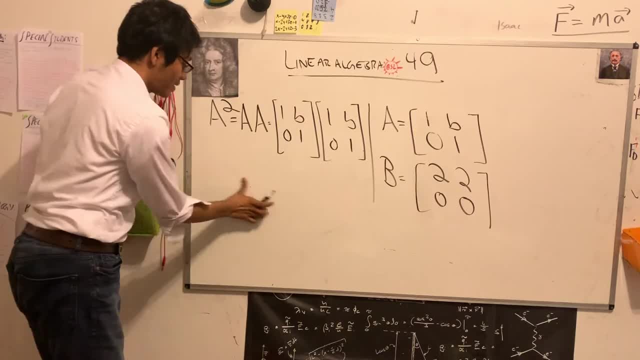 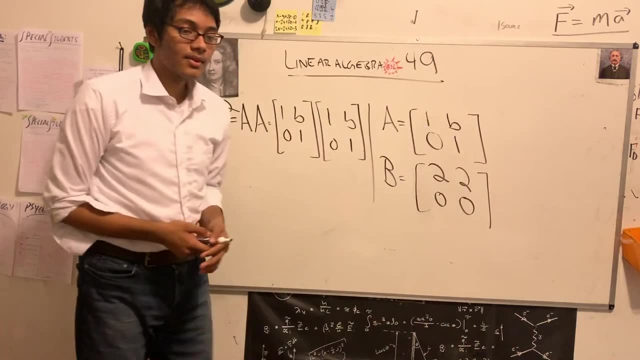 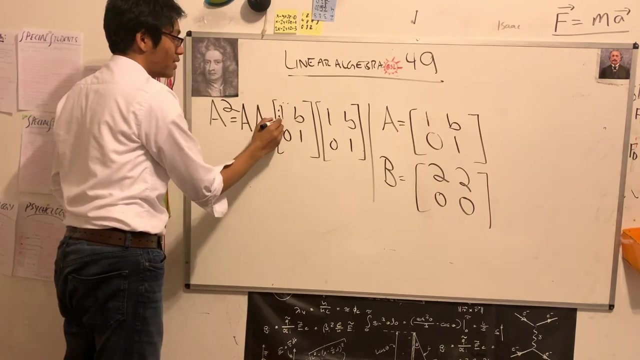 to start with the roll and a column. so i have three different options. what option do you guys want? dot, product rules, columns. i did the column. i did the wrong way, so it's wrong way. okay, alex. rowing- okay, row away- okay. so rowing means let's look at the first row. first row tells me. 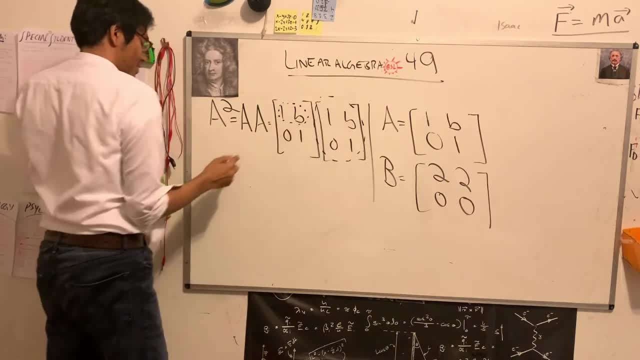 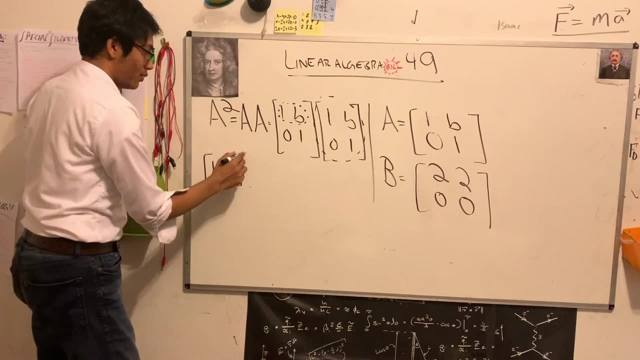 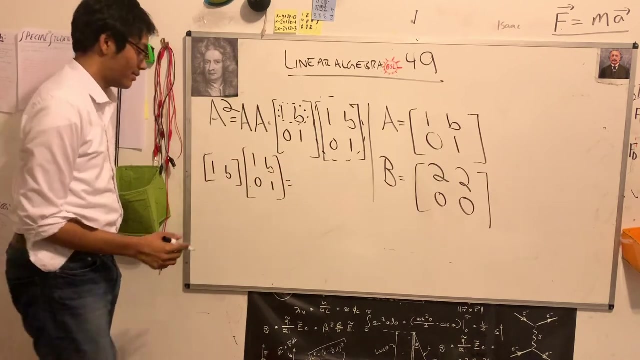 i have to multiply this row by the entire matrix, okay, so hopefully this is easy for you now, or if it's not easy, at least elementary one, one b, times the entire matrix, right? so what happens when i multiply a row by a matrix? this tells me i want one of the fast row. 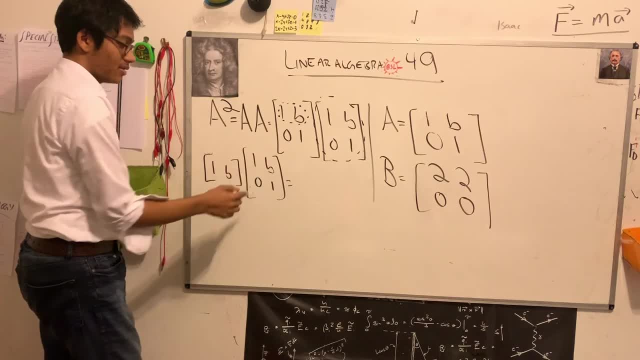 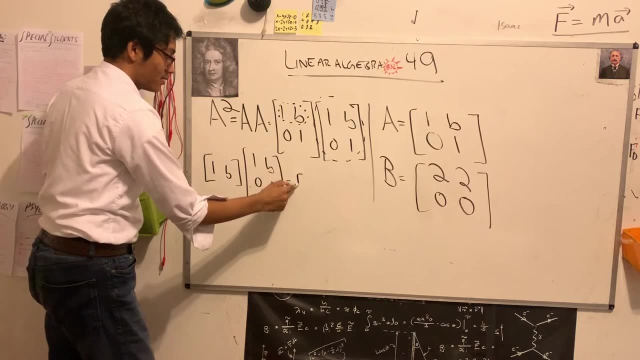 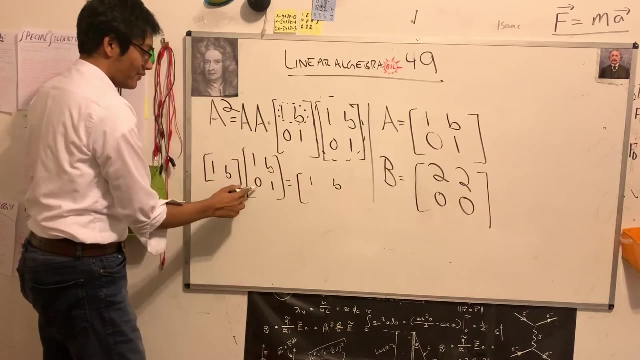 b of this, b of the first row. right, yeah, wrong. i want one of the first row, b of the second row. so that means i'm going to get what one of this is going to be one, okay, one, one bp, and b of this is gonna be zero b. 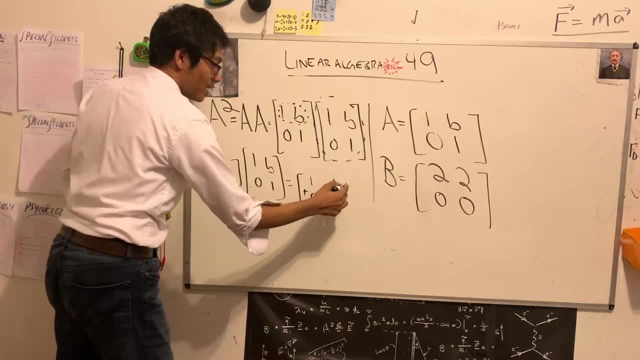 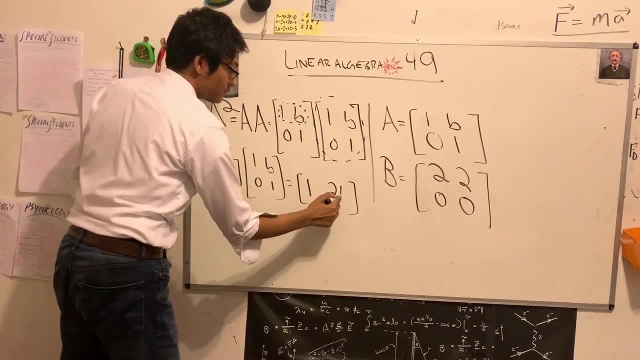 zero b. but this is not a matrix. i have add these two rows up, okay, so 1 plus 0 is 1, B plus B is 2B. oh, that's how you got. that's why the first row of a squared is gonna be 1- 2 B. but we still have to. 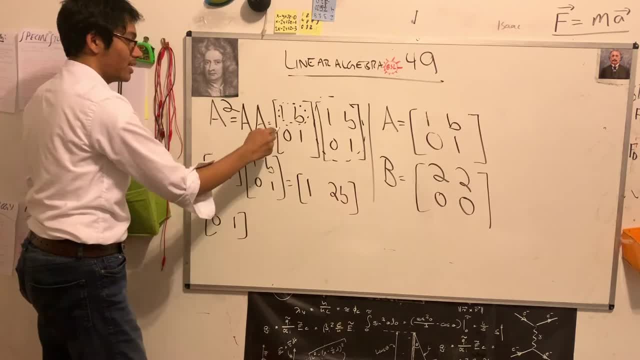 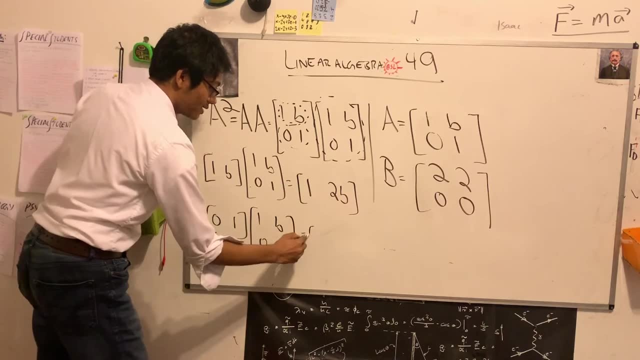 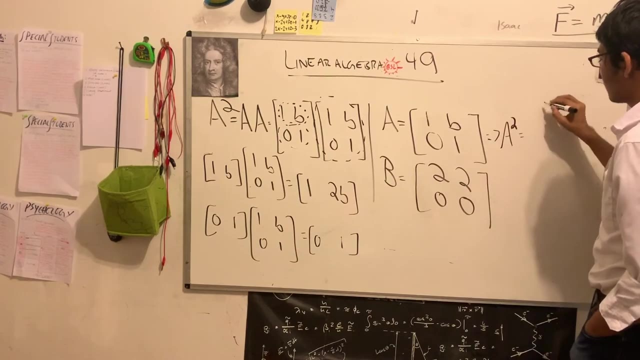 find the second row. okay, so take the second row. yeah, so you just gonna take the second one. that's all I say right now. I know what a squared is. a squared is what a squared is equal to 1, 2 B. 1, 2 B. what is 0 1 0? 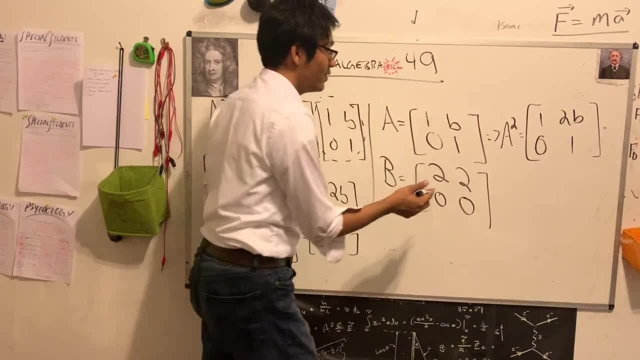 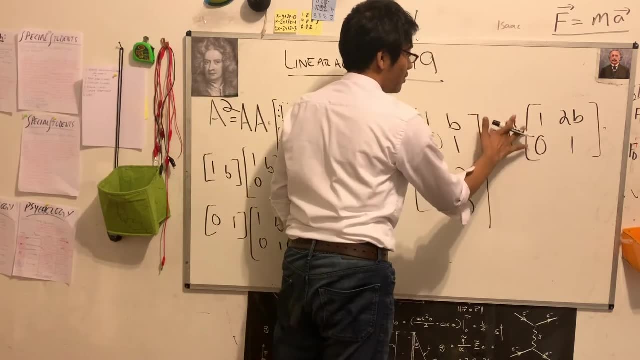 and it turns out, if you keep doing this, if you now, if you're trying to find a cute, okay, why am I writing again? if you try to find a cute, what do you think is gonna be? yeah, 1 to 3 B, if you're finally, fine, very. 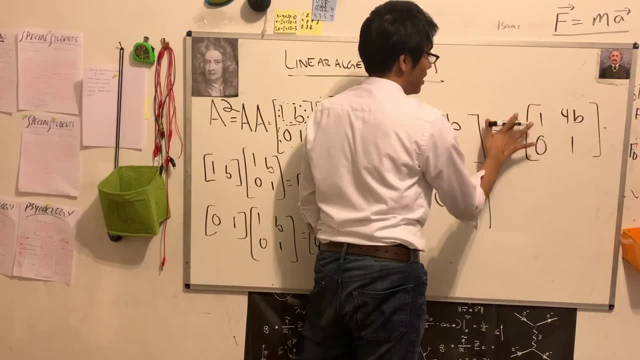 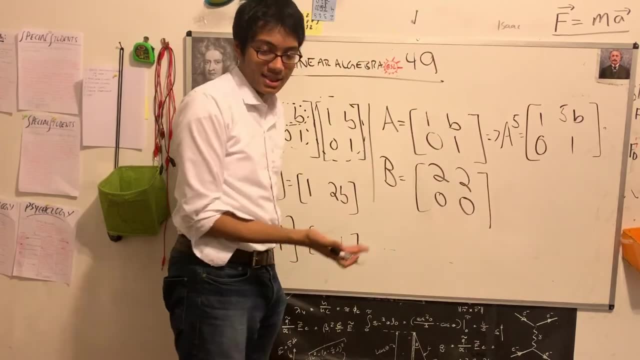 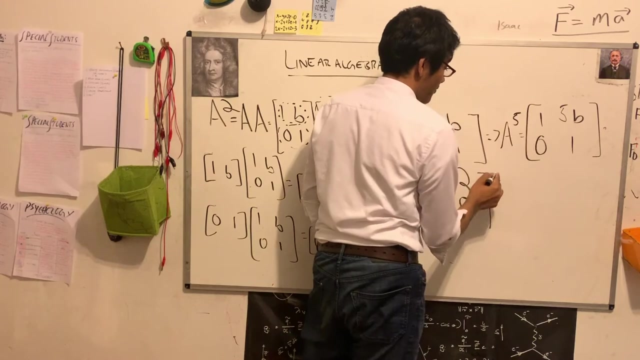 fourth, what is it gonna be? one, four b, wow, army. So the power become the coefficient of this. constant now, In a very magical way, Variable now, but constant later. Yeah, Now I'm going to ask you to generalize. okay, If I have A to the N, what will it be? 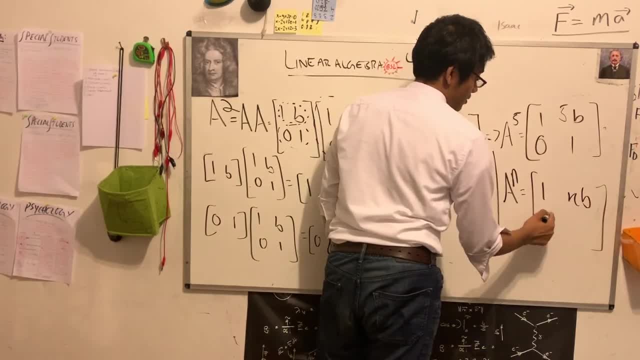 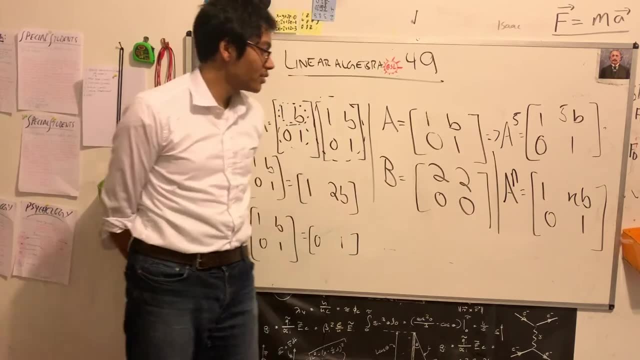 N, NB, NB, NB, yeah, yeah, yeah, Right. Okay, Mr Andreas is left doing the y's, Yes, But now what we're going to do is take a look at yet another example of matrix powers. 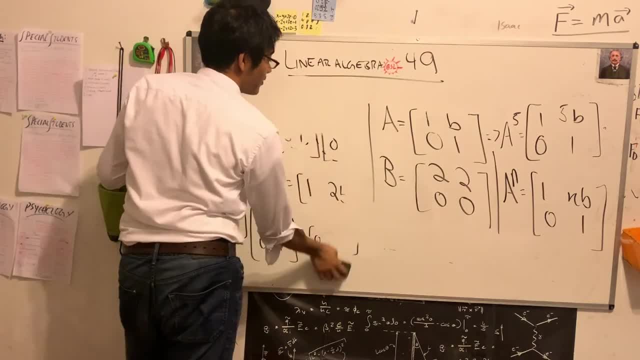 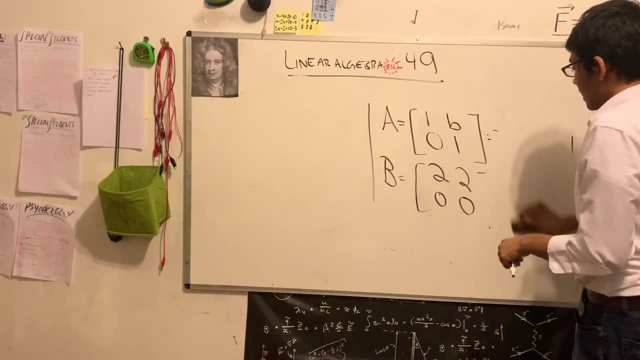 And that's going to be matrix B, okay, So let me erase all of this. So, what is my matrix B? Well, my matrix B. I've written it right here, But I'll write it very nicely once again, Okay. 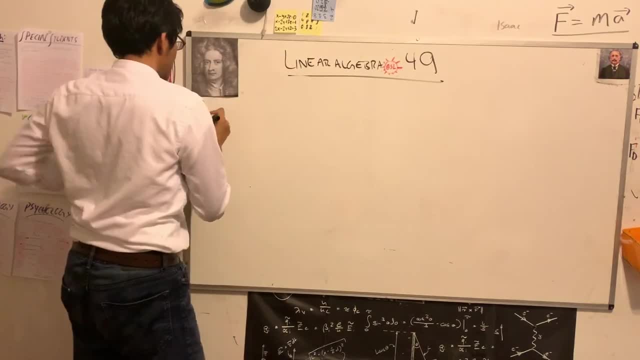 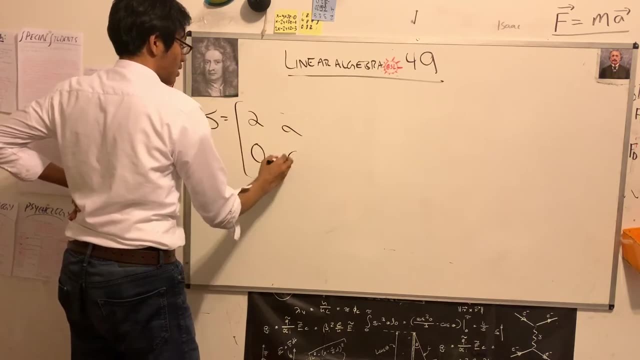 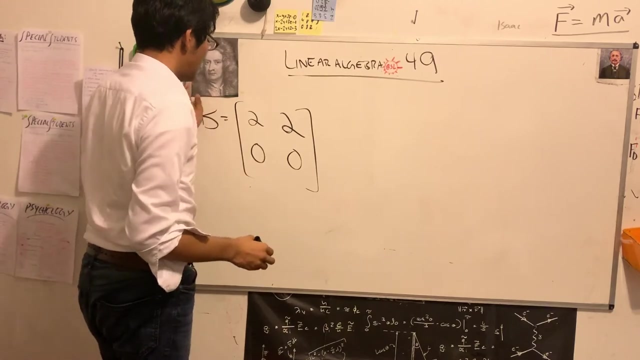 So it's going to be 2200.. Sort of like this: B is equal to 2.. 2,, 2,, not none. Okay, Hey, what about getting back from the right? Yeah, So now I have a new matrix called B. 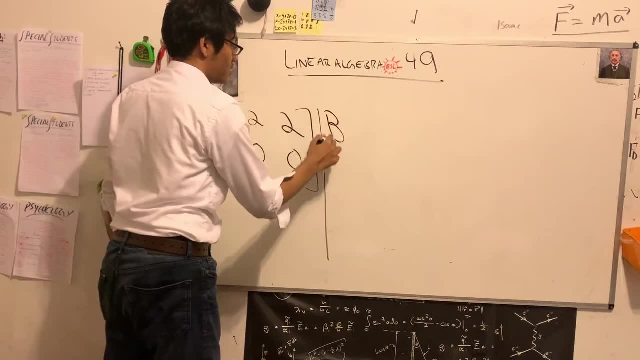 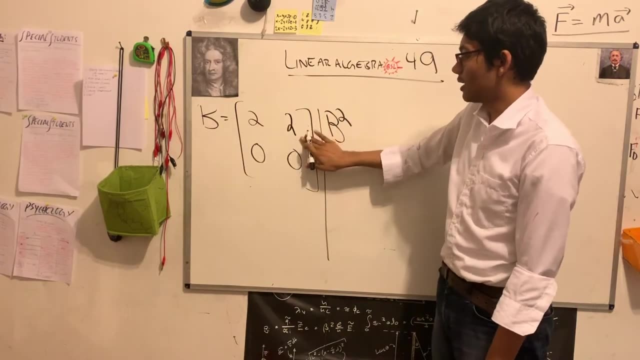 And I want to find its power. okay, So, before I do any math, before I do any math, I want you to make a prediction, Because, by the way, I didn't do this, But I will also myself make a prediction. 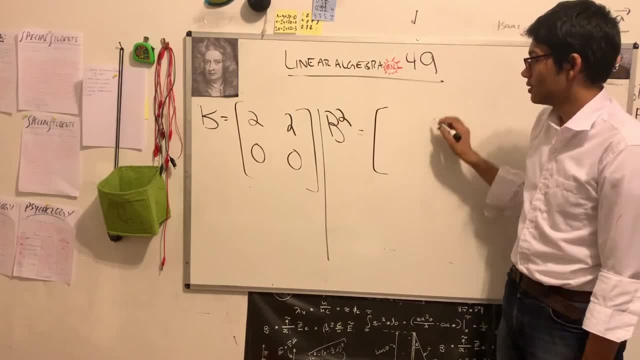 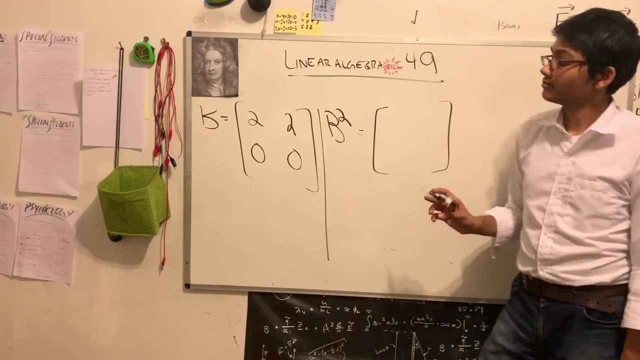 So who wants to make a prediction? What is B squared? Any idea? Yeah, You can do it. Oh, no prediction, No math. Oh, One minute: 2, 4, 4, 0, 0.. 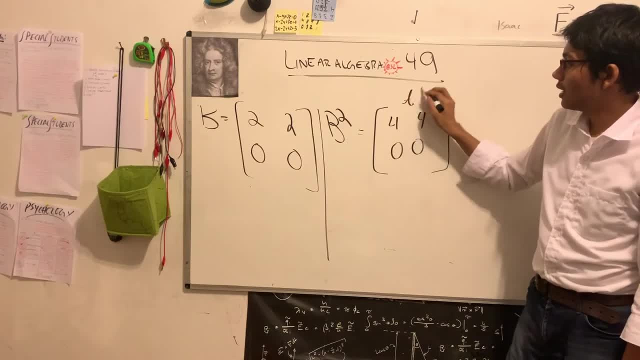 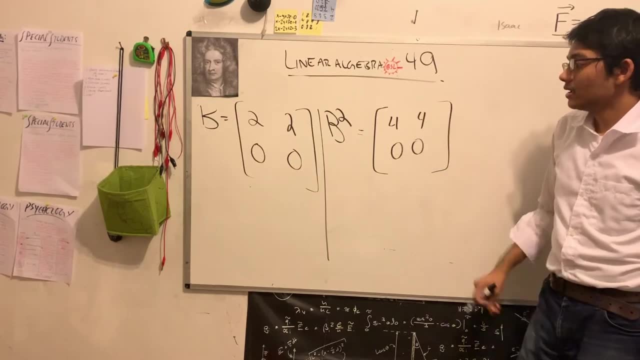 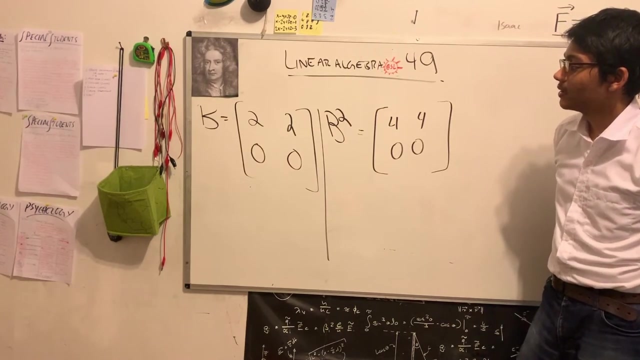 Okay, that's. I'll call that Alex's prediction. Yeah, I agree, I agree, Okay. so okay, That's your prediction. You know what I predict? This is wrong. This is wrong. Let's see, I want to do it in my head. 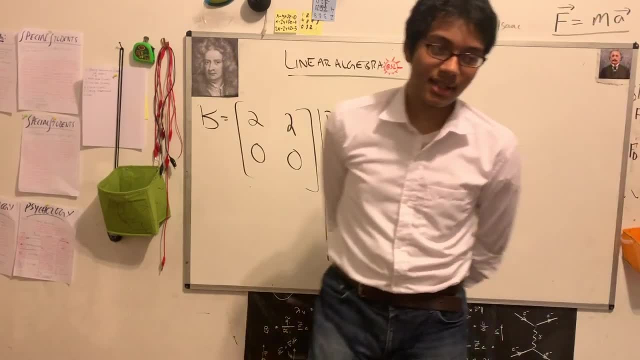 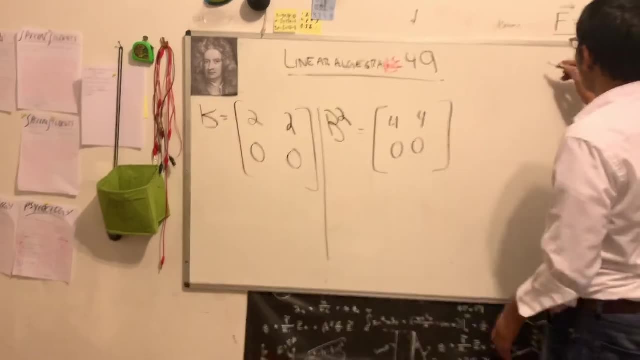 Okay, Boom, boom. Okay. I'll also agree with you guys, Because I have no other common sense way. So what we're going to do is we're going to multiply it out, Because we don't know if this is true or false. 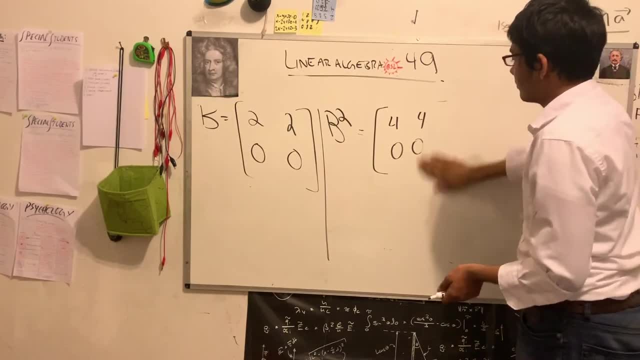 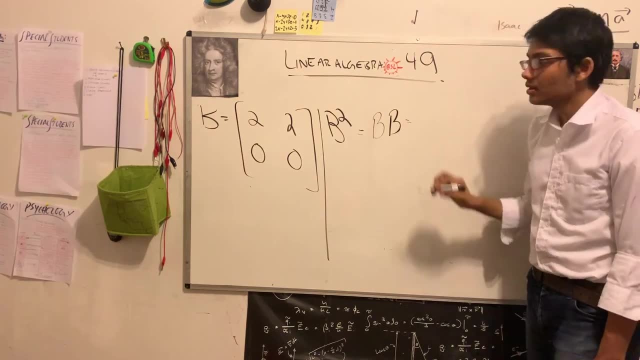 So I'll keep your prediction in the corner, okay, So B squared is obviously going to be B times B, right, Yeah, yeah, So that's going to be 2, 2.. So let's write it. 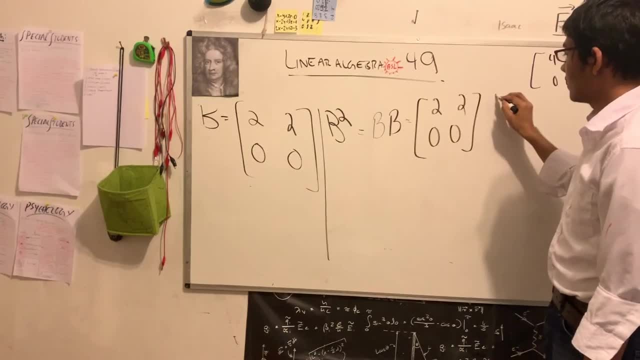 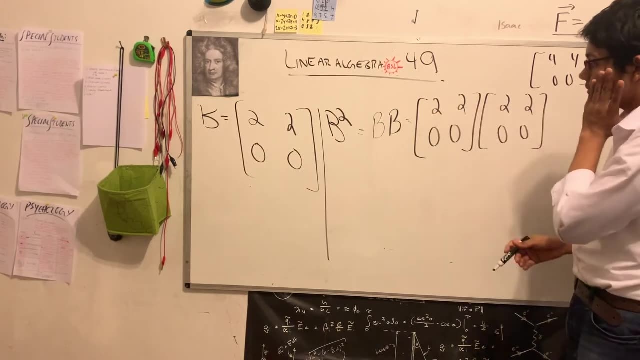 2, 2.. So that gives us 8.. So that gives us 8, 8 for the first one. But wait, wait, wait. So I have to multiply. Okay, you know what I'm going to do. 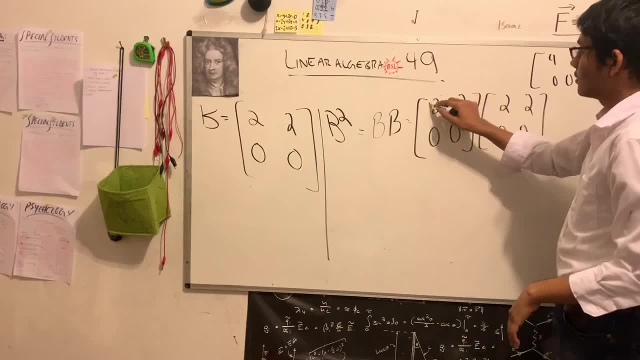 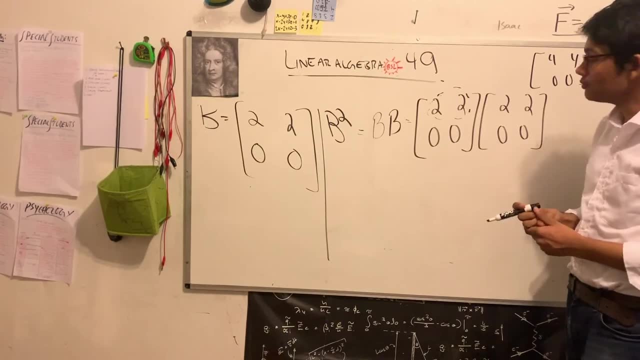 I'm going to do the row weight, The row weight. Yeah, you want to know something smart? No, you can add the two things in the first row and then multiply it by the second row to instantly get it. Yeah, yeah, but let's do this. 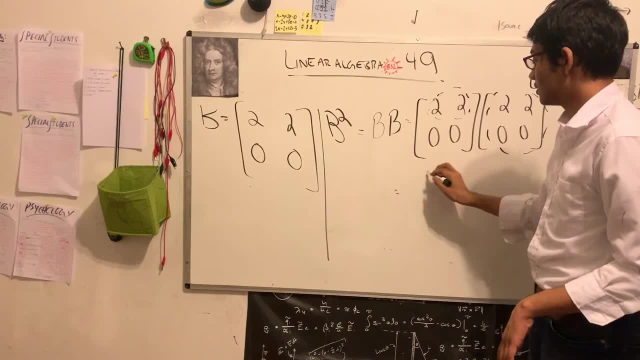 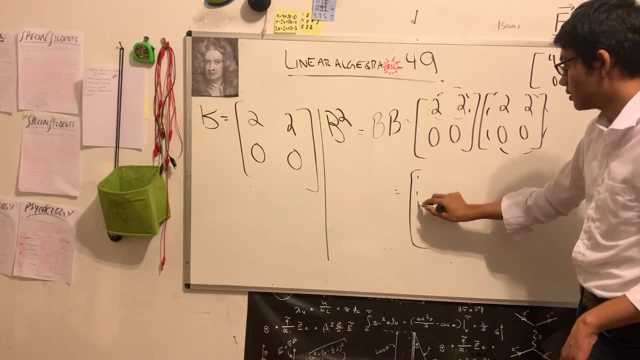 So 2 of the first row is going to give me what 2 of the first row is going to give me. 2 of the first row is what Is 4.. 4. Uh-huh, So sorry, I'm working in the first row. 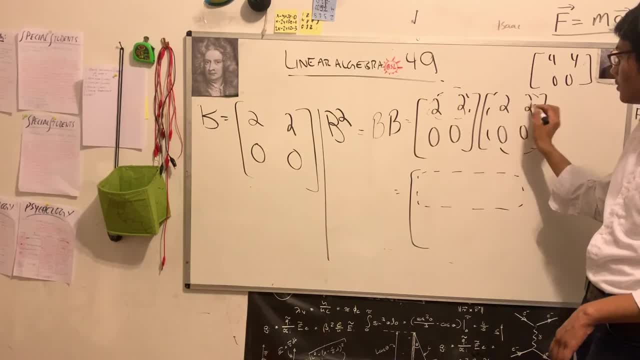 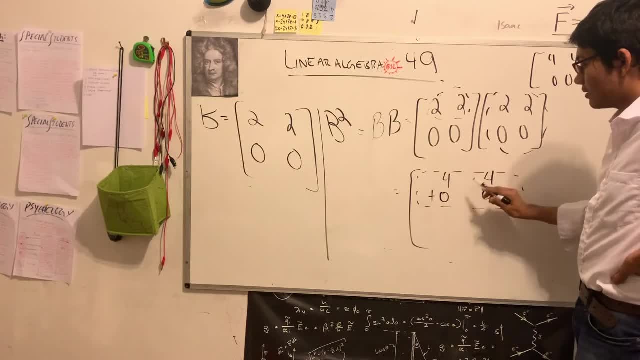 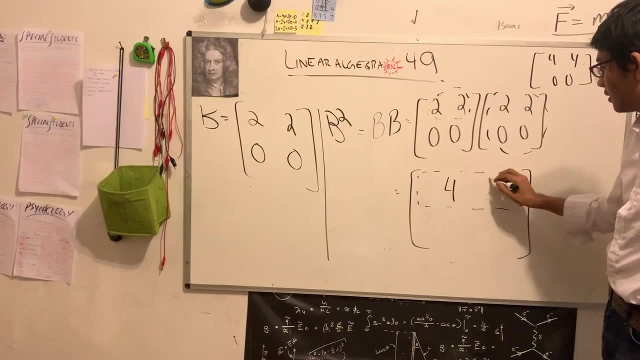 0, 0.. 0, 0.. So if I add these up, I'll get that the first row of my product is what? 4, 4.. And 0, 0 will just set the whole other matrix to 0.. 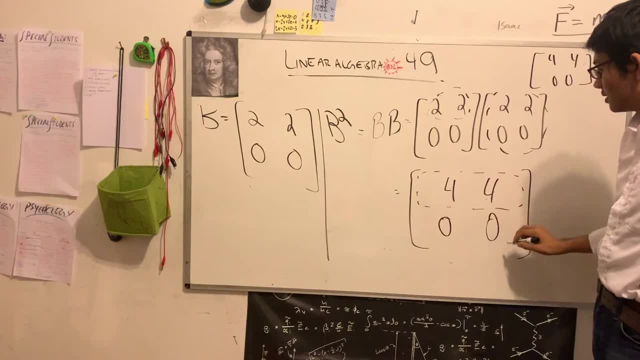 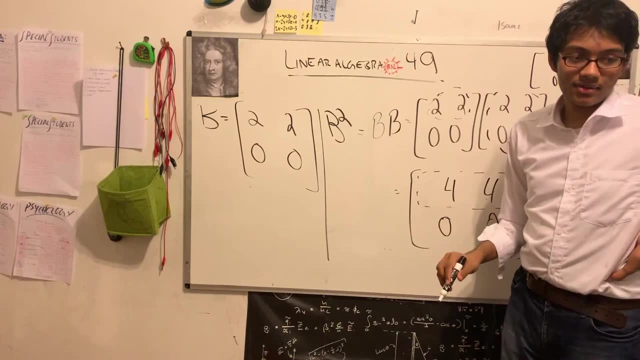 Oh, so you were right. Is that, was it right? Yeah, Ah, prediction meets reality. But now, Now, now I'm going to B cubed would be 6, 6,, 0, 0, right. 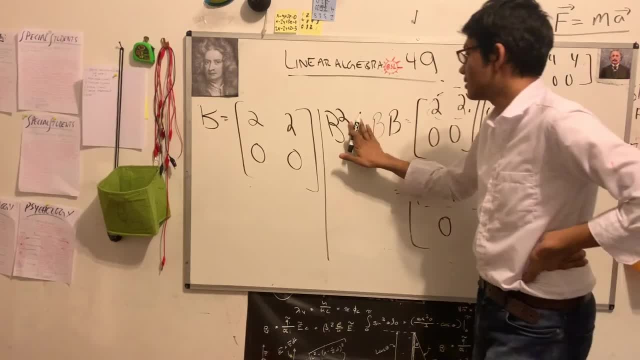 Now I think it's 6, 6, 0, 0, but I'll ask you to make a prediction once again. So this time I'd say 6, 6, 0, 0,. I agree. 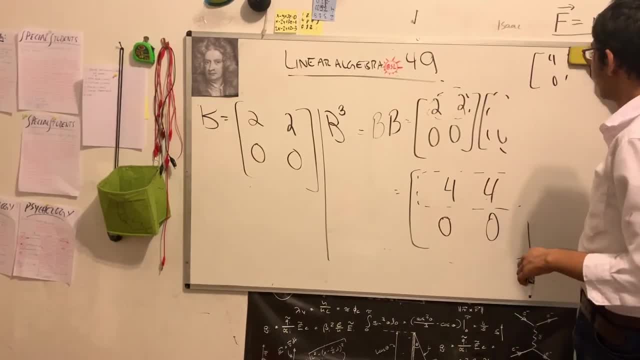 Let's ask Alex what he thinks B cubed should be. Do you think it's 6, 6, 0, 0?? Uh, 2 times 2 times 2, 8.. That's 8.. So 8, 8, 0, 0.. 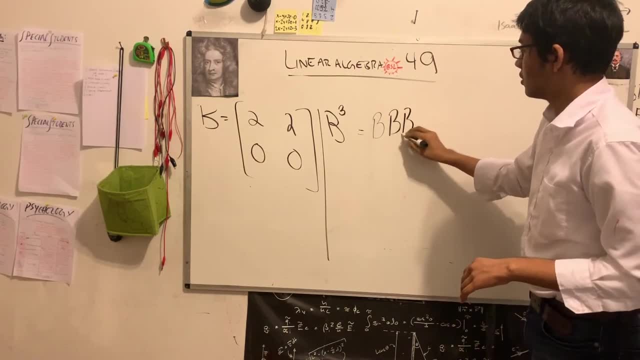 Okay so, But remember the pattern It was, it was the co-option. It was the co-option, not the actual one. So, Alex, what do you think? He said? 8, 8, 0, 0.. 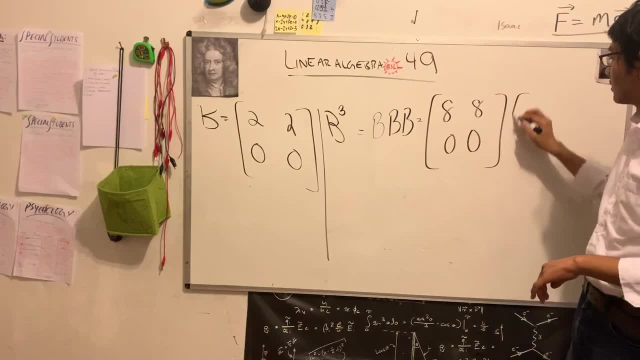 He said 8, 8, 0, 0, what do you think? Uh, 6, 6, 0, 0.. Well, I'm afraid I'm going to have to side with Alex on this one. 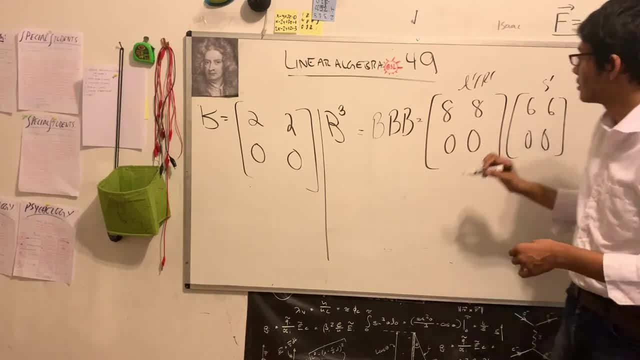 Uh, so let's see who's right Ready. Okay, I will do it. The odd one, I will do it. Oh, no, no, no, you'll come up for the existed, Okay. So yeah, yeah, okay. 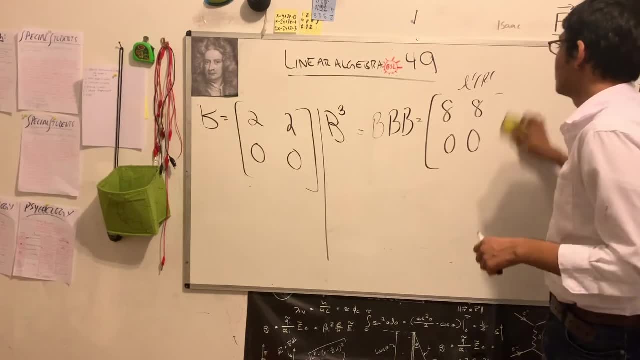 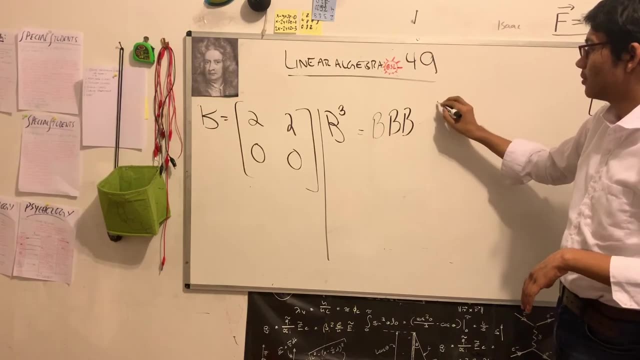 So let's see how it works. okay, Uh, okay, Okay, let's get, Let's start it. So B B B, So B times B times B is going to be what: B B B. 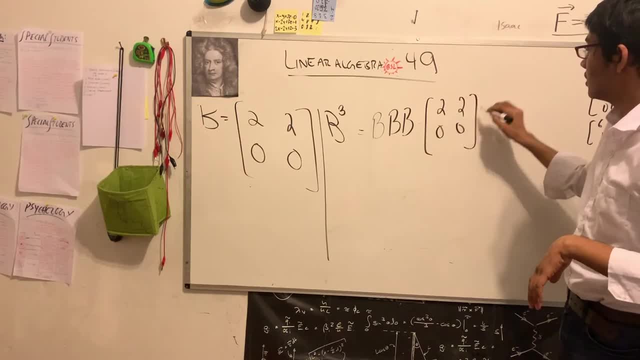 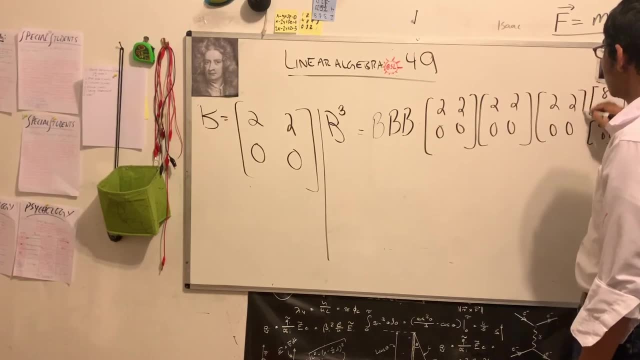 So we have to write this in a nice way, or it's not going to fit. So 2, 2, 0, 0, 2, 2, 0, 0, 2, 2, 0, 0, right. 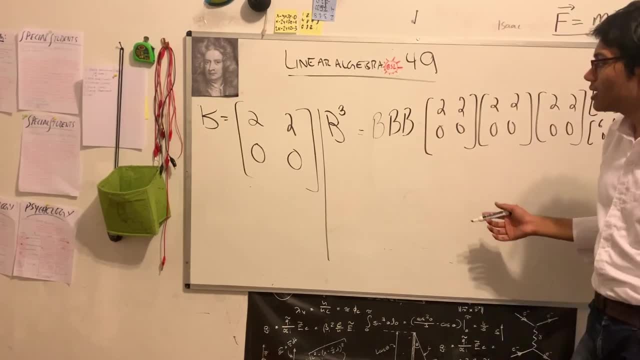 Oh no, it's 8, 8, 0, 0.. But, but wait, We already know what B squared is right, So why do we have to waste time doing this one? We already know this is what. 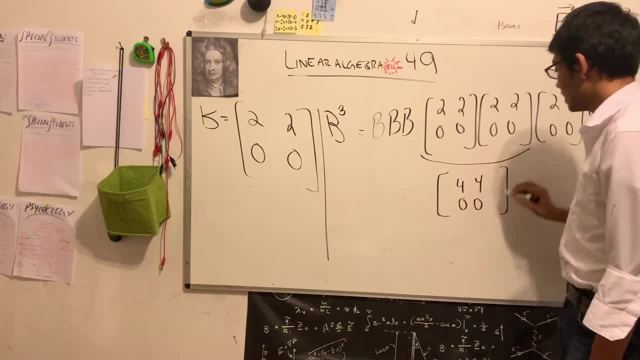 4, 4, 0, 0.. 4, 4, 0, 0.. Okay, that makes out like Okay A little bit easier. Oh, it's 8, 0, 0,, 1,, 2, 8.. 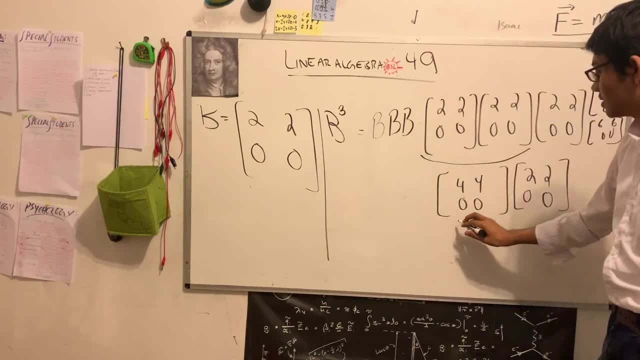 And now it seems like one of our students already realized his mistake, but let's do it up, Okay. So what would our first row be? So, Oh, 4 times 2 is 8.. 4 of the first row. 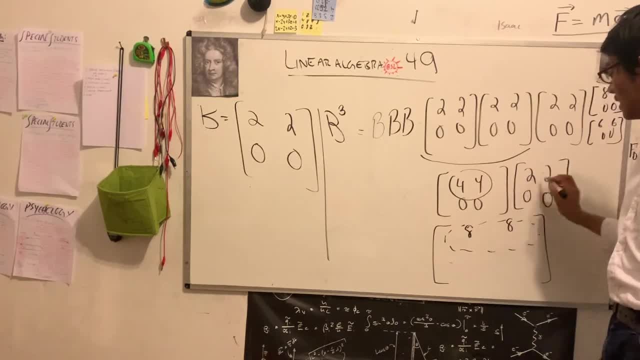 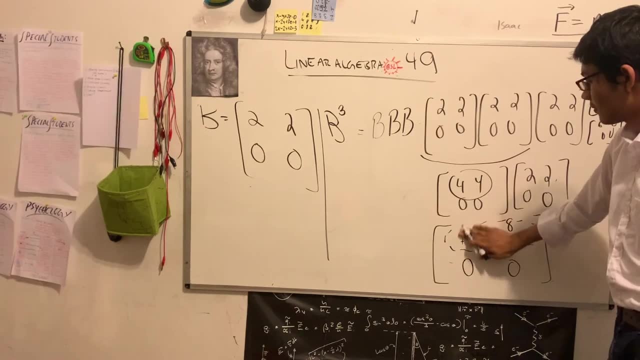 I got it. 4 of the first row is 8, 8.. 4 of the second row is 0, 0.. And of course, this is just 0, 0.. But, but, but. I have. 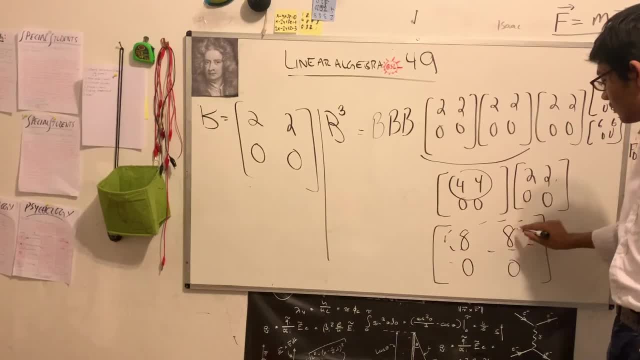 Yeah, But um, That doesn't follow the pattern we saw in the do-now. That's right. Can you tell me why? I don't know. Is it because the do-now there was the identity Number one? the do-now was an identity matrix. 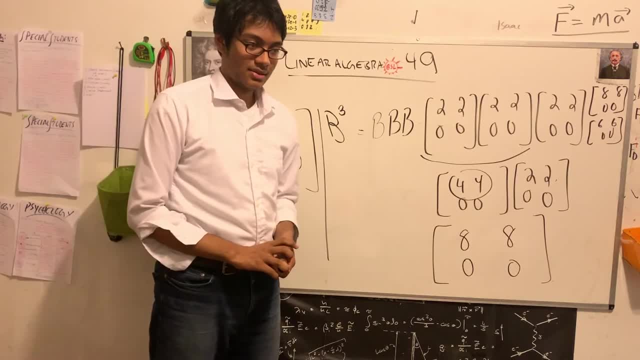 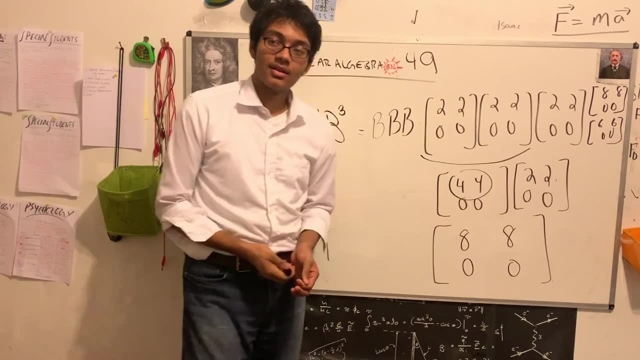 Number two: the do-now was a snow. It was not a symmetric matrix: A snow, I think A snow, I think it, it I guess it do-now, because there was B and 2B. B and 2B, yeah. 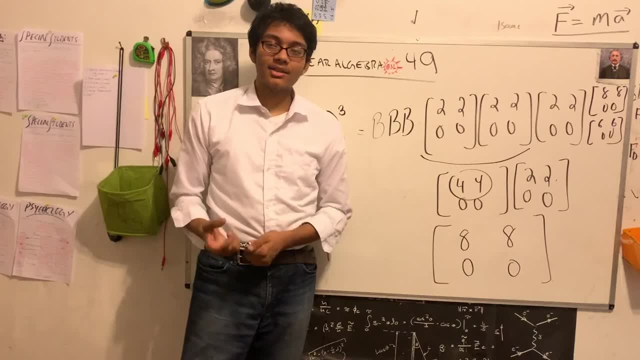 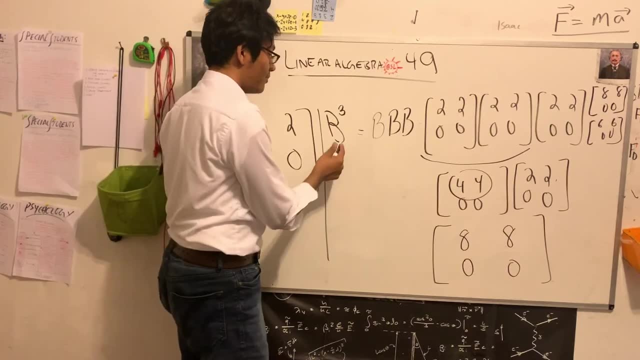 Um, maybe it was identity matrix. that's why Identity matrix is special, because it's, it's, uh, it's almost symmetric, It's half symmetric. you can say: Um, this is not even symmetric at all, or even half symmetric. 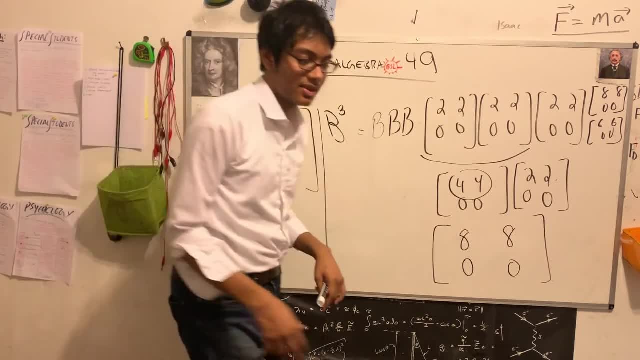 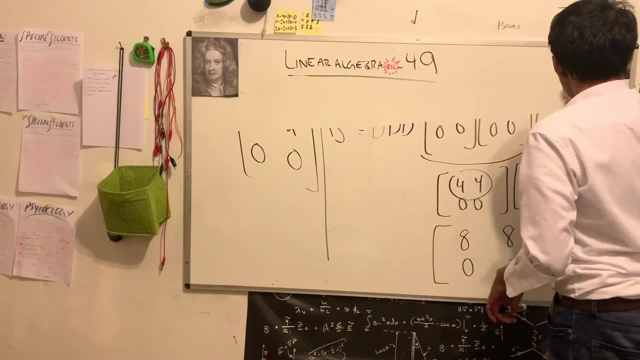 We'll talk about symmetric matrices later. but, Oh, but in the regular definition it would be symmetric. Um it? no, Because there's two zeros on each alley. No, that's not how. Oh yeah, regular definition: it is symmetric. 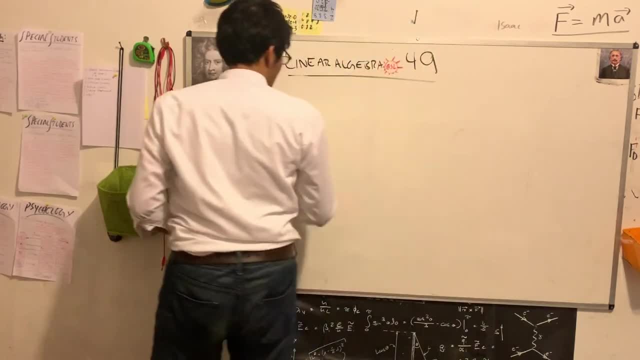 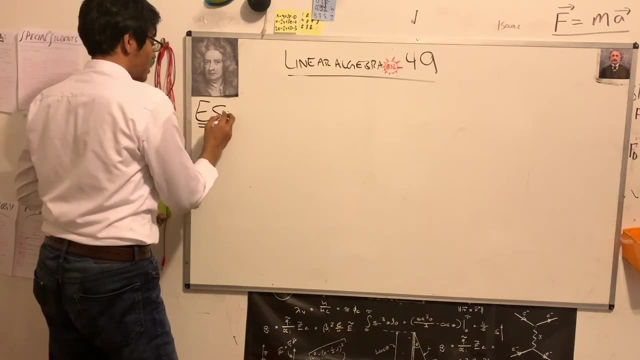 But in our do-now it was not symmetric, Yeah, because, Uh, I'll call it half symmetric, half symmetric, okay, Uh, now we're gonna move on to: uh, um, we have existed, and that is this. 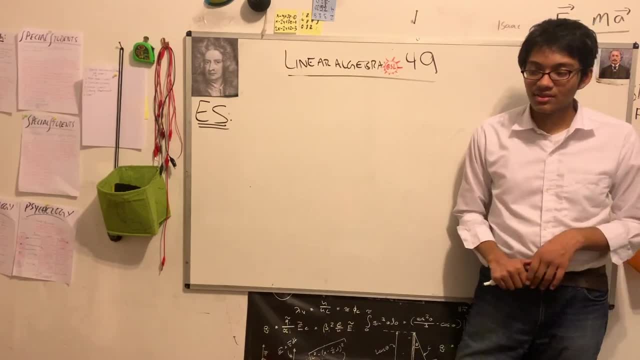 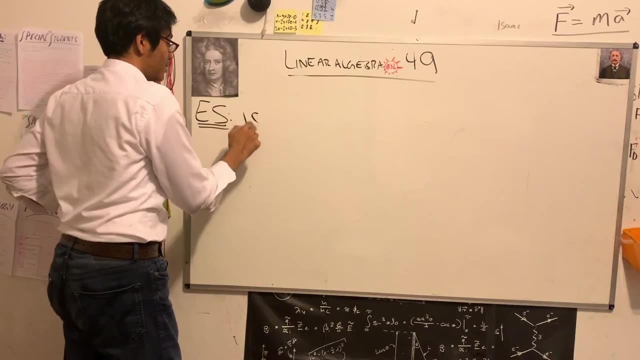 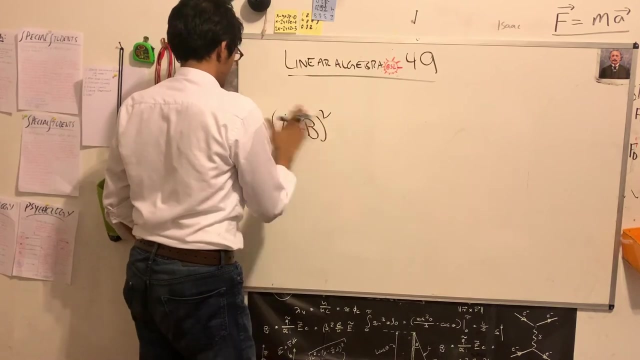 Oh, we are one, It's gonna. it's gonna test your, test your ability to kind of retain concepts And um, okay. So here we go. Okay, Um Half existed, Oh, A, So you know what? 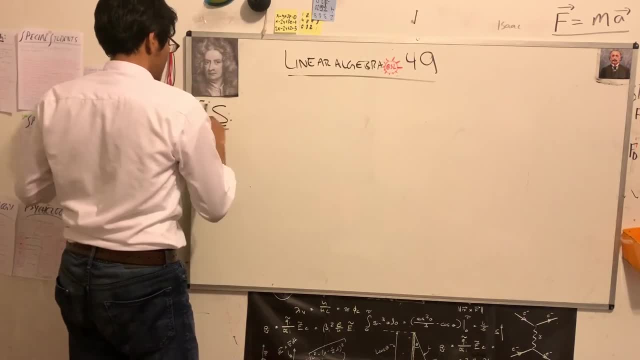 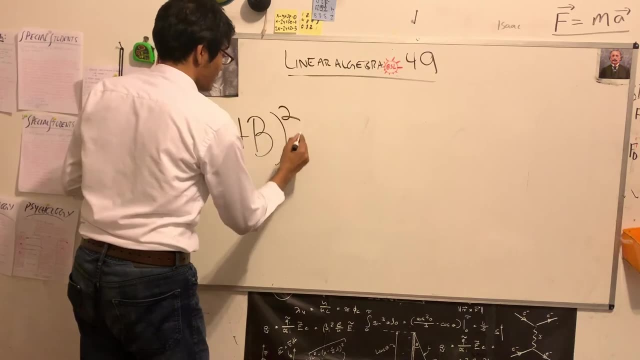 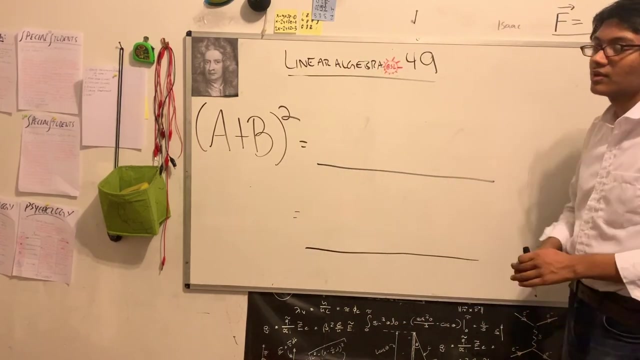 I should probably write it big because people don't see it. Okay, So here it is. I'm an expert at multiplication and addition for for matrices and I'm the speed one. this: So B plus A squared. So who wants to come up and try? 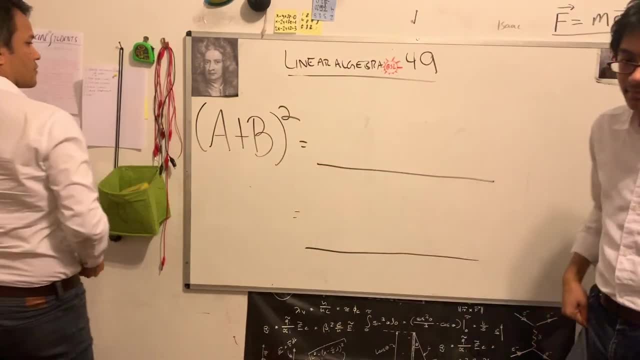 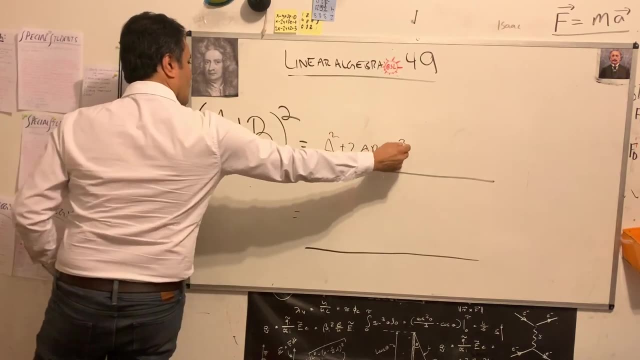 Um, Wait, what are the matrices? What are the matrices? It's general, It's general. And uh, next lesson we're gonna, I know this, but uh, what do you learn through this? Oh shoot. 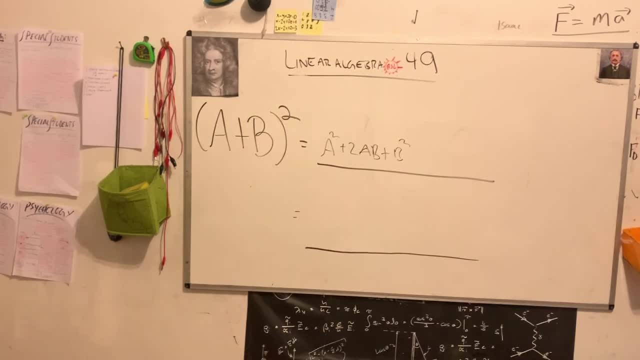 He did the binomial way, Okay, And so I'm saying: would you like to? uh? Why are you calling me professor? I'm sorry, Uh, instructor. Oh, Let's go. Let's go ahead. You're handing the class to me now, huh. 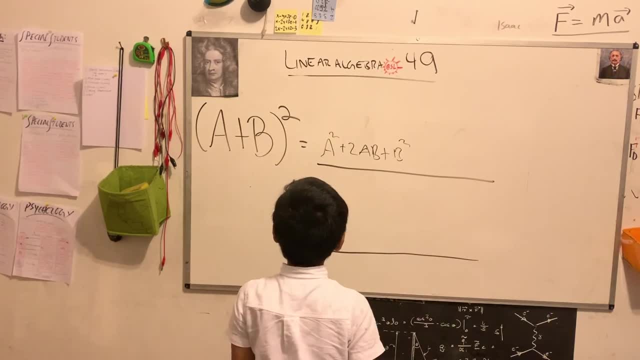 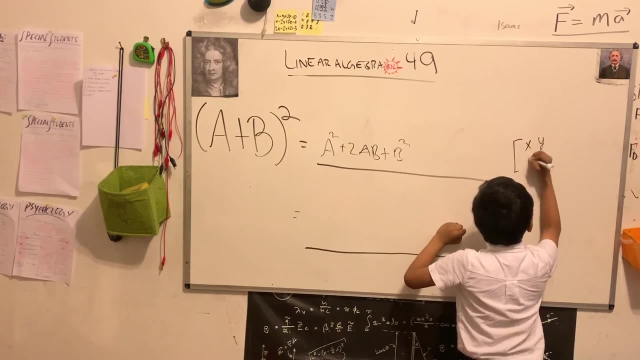 Okay, So what I think? um A plus B squared, So let me just test this out with: Oh, whoa, whoa, whoa, whoa, whoa. We don't have time for tests, Okay. 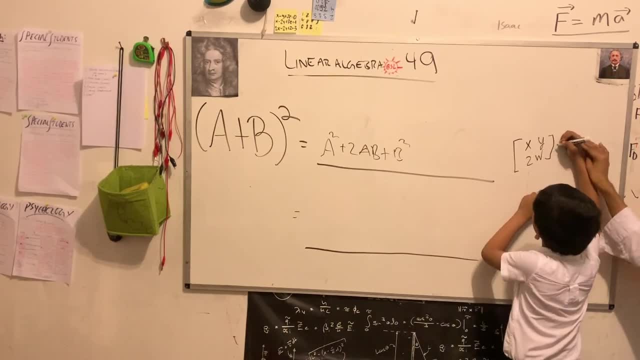 No, no, no, I'm an expert. No, no, no, no, no, no, no, I'm an expert. Um, we don't have time for this. No, Just make a prediction and you're set to. 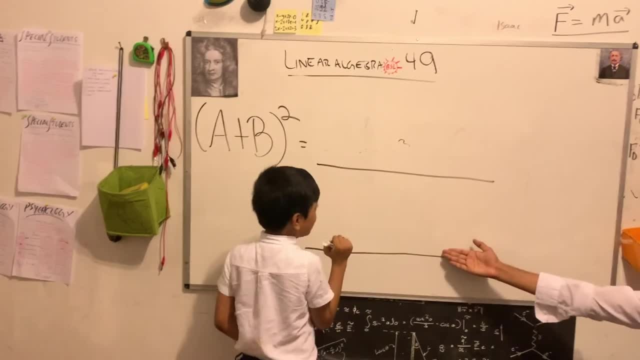 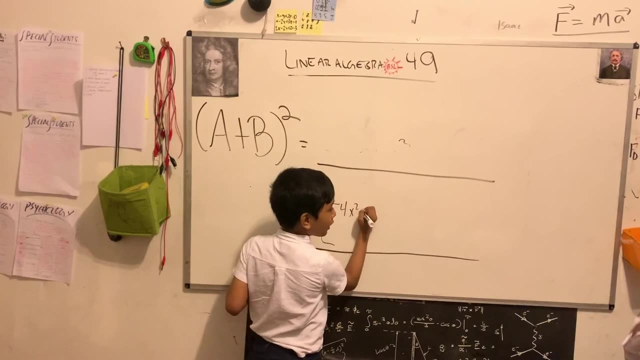 That's what we do in math: Make a prediction. I'm No, no, write your answer on this line, Okay, Uh, so, uh, I'm, uh. can you tell me anyway, four X squared, Oh. 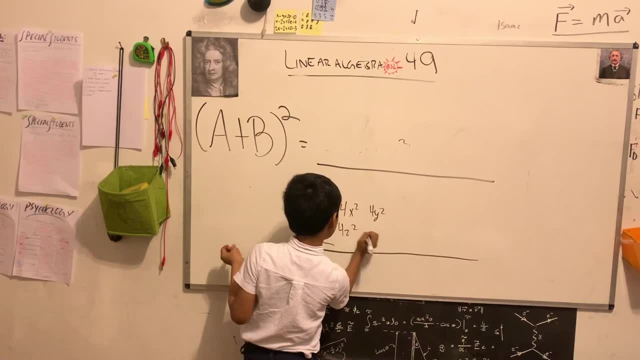 For A Y squared, Uh, four Z squared. Where did the four come from? Oh, Four W squared, Okay, Okay, I'm using these variables to generalize, Okay. So let's see, It can be any uh number. 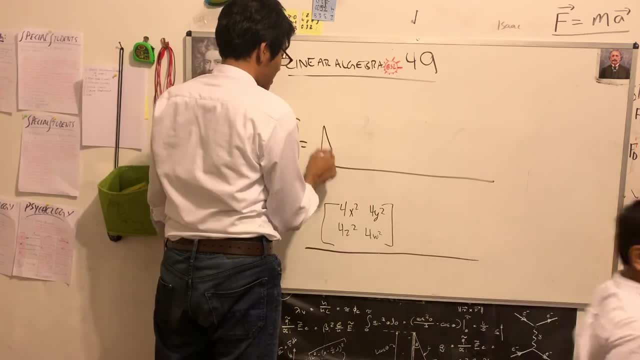 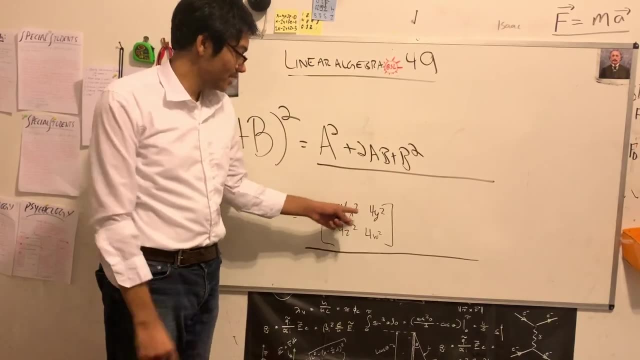 Uh, get this, get the talk, Thank you. So Alex predicted A squared plus 20B plus B squared, And Isaac, uh, predicted four X squared, four Z squared, four Y squared, four W squared. And here common sense wins out. 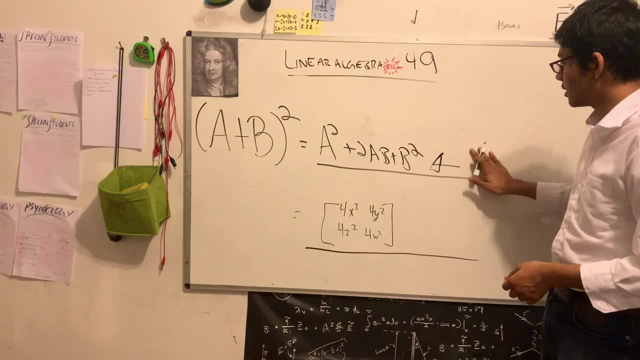 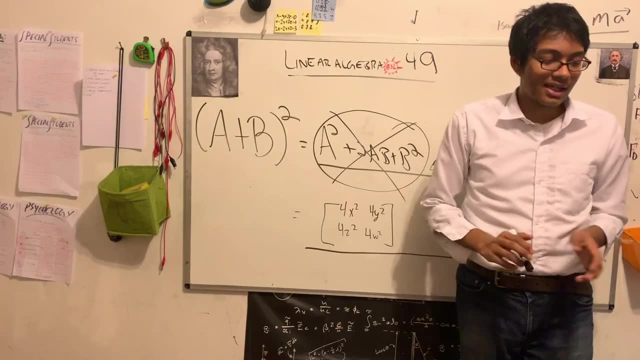 Uh, the answer is indeed. uh, no, it's not. This is: this is a common-studio misconception, Right? This is completely bullshit. Okay, A plus B squared This. this is my mobile one. This isn't algebra. 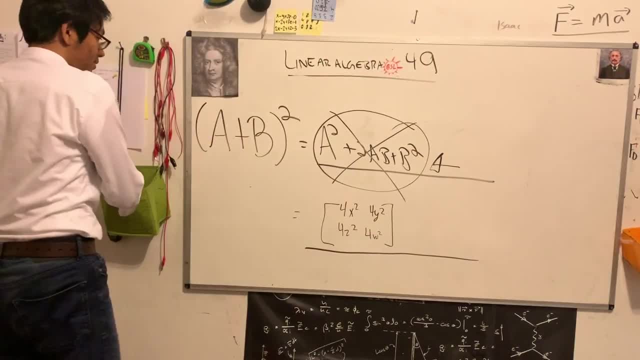 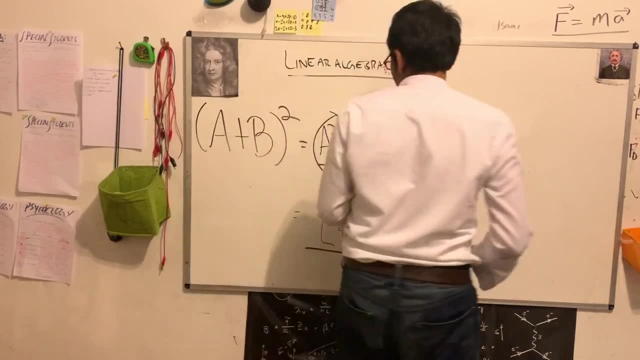 This is linear math. Oh, This is wrong. Okay, Oh, Why? This is like saying that, this is like saying um, What So linear means in algebra? No, no, no. Doing this in linear algebra is the equivalent of doing this in regular algebra.